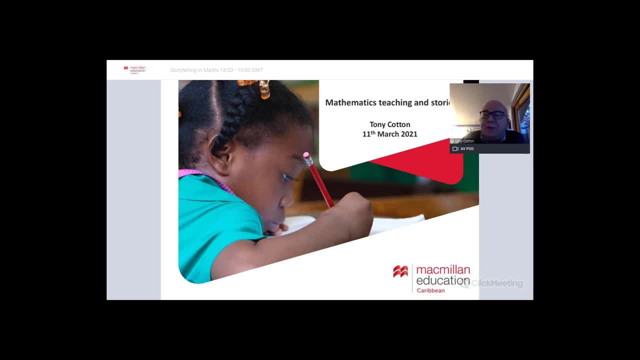 where Leeds is, But it's wonderful to have so many of you here joining the webinar. This is the second one today. We had a great time earlier on, About four hours ago, we ran this webinar the first time through and people seem to enjoy it, So I hope you'll enjoy it. I hope you'll enjoy it. 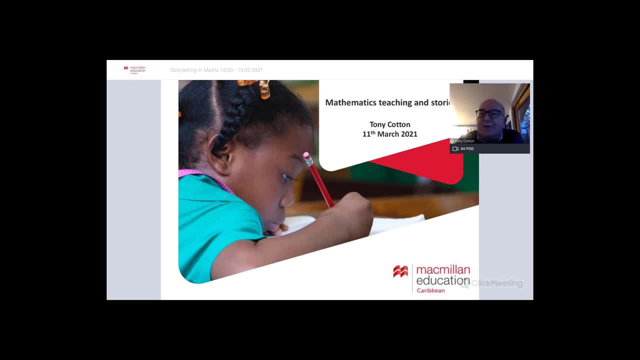 As much as the participants did earlier this afternoon And I hope I enjoy it as much as I did earlier this afternoon as well. I'm sure I will, And I've really enjoyed thinking about mathematics teaching and stories. When Macmillan asked me to to plan this webinar, I very much enjoyed thinking about it And 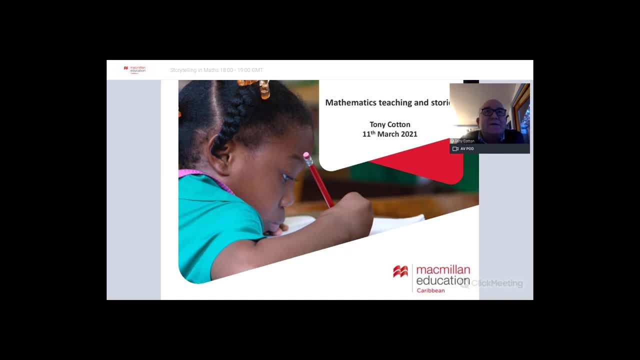 one of the things I've enjoyed is trying out all of the activities that I, that you are all, introduced to with my, with my grandchildren, just to make sure they were fit, fit for purpose. And, as well as being a mathematician and a mathematics teacher, I read all of the time. I'm a, I'm an avid reader, And it's been so it's. 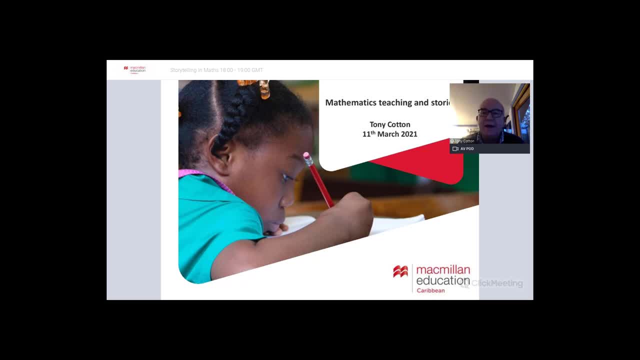 been a treat to put those, to put those things, things together, And I'm a member of a book group that we read books together- I'm sure many of you are in in similar groups- And we read themes, And we read themes. 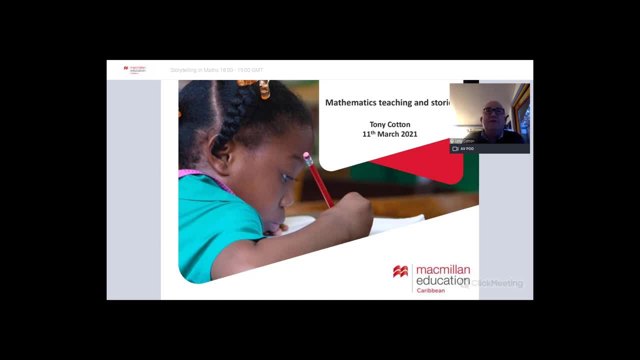 we tend to read seven or eight novels- mainly novels- around a theme Each time. Three themes ago, the theme was around mathematics, And that was how mathematics is involved in in some novels And currently where our theme is Afrofuturism. I don't know if you've heard of Afrofuturism as a genre. It's. it's science fiction, but 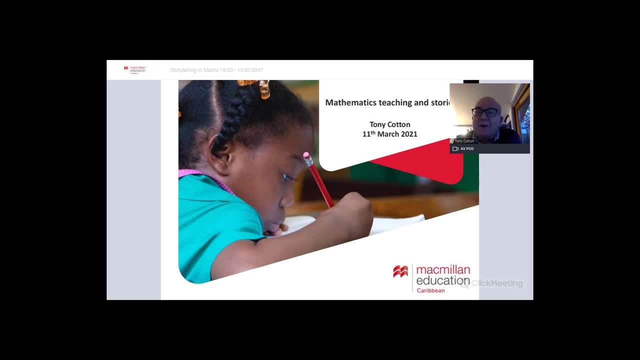 written by writers from Africa and from an African American writers. In fact, Beyonce is seen as somebody who's an Afro Afro futurist because of her, particularly her last album, which was very much kind of quite science fictiony. And, of course, 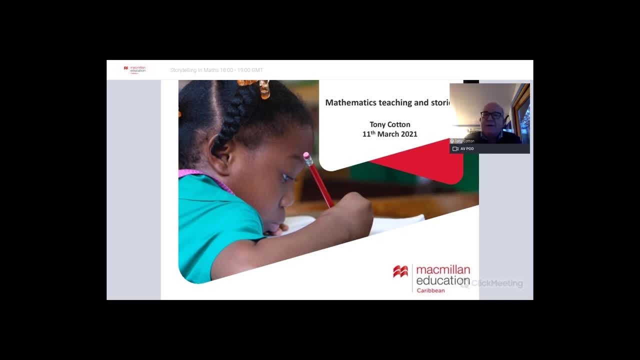 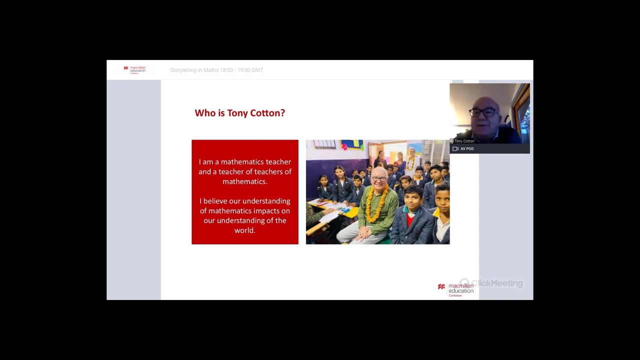 there's lots of mathematics in in science fiction novels, But we're not talking about science fiction today And we're not talking about maths in novels. We're talking about creativity and how we can use stories to to teach mathematics. I know that several of you attended the previous webinar. we 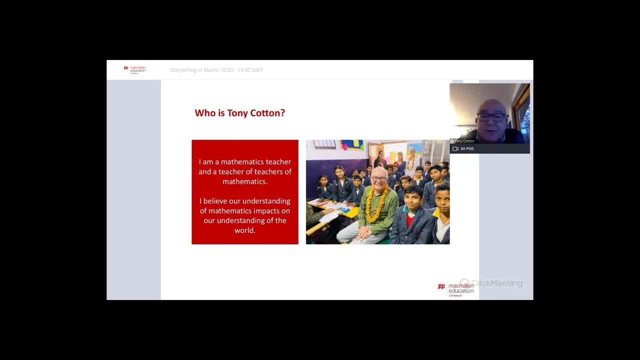 looked at mathematics in the real world. There's a real storm breaking here. you can. you may start to be able to hear rain. It's very windy and very wet, So if you can hear the storm in the background, that's actually a storm in England, not, not? not as bad. 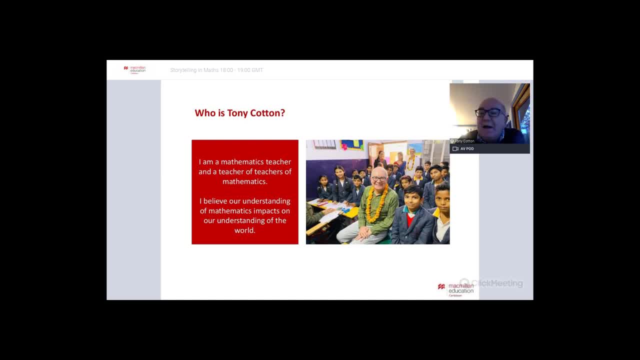 as storms that you get, but fairly bad for storms here. But I'm sure I'm sure I'll survive And I'm only about 10 yards from my house if it gets, if it gets too damp. Anyway, for those of you that were in the last, the last webinar, you'll 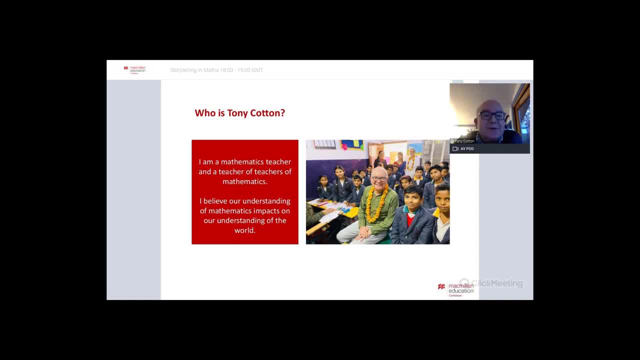 remember that I use that, say those same phrases to introduce myself. I said I'm a mathematics teacher and a teacher of teachers of mathematics, And I do both of those things. So I still teach mathematics. I teach mathematics to children in schools whenever I can. Obviously, that's been limited in. 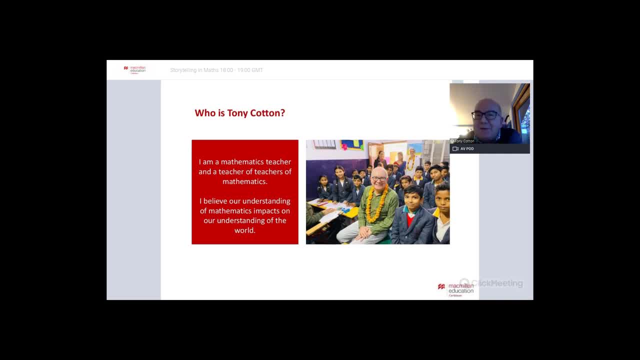 the last, the last year, I teach mathematics to my two grandsons During lockdown. that's been. the highlight of my day has been my zoom, zoom lessons with my grandsons aged eight and three, And I'll talk a bit more about them then later on, And I'm also 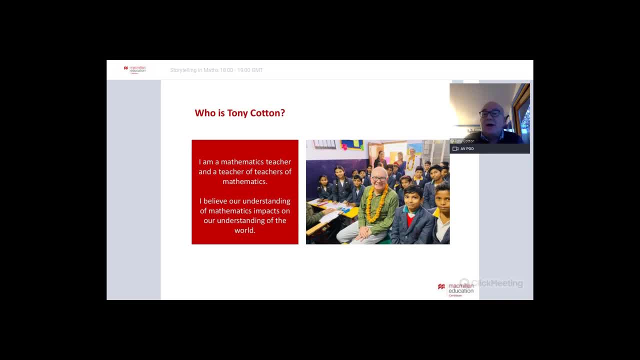 involved at the moment in teaching mathematics online to children in refugee camps in Greece. I think one of the fascinating things about about the last year and about learning to teach online and learning to to teach remotely is how quickly we've adapted to new ways of working. 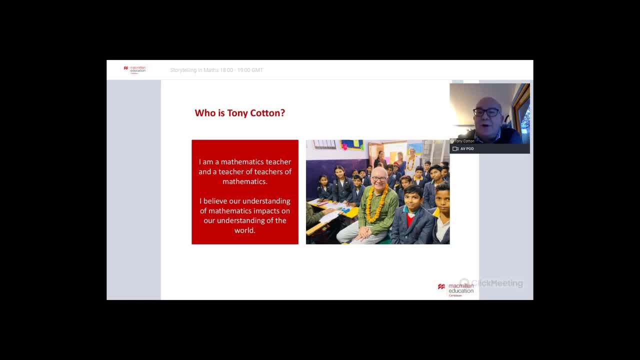 And in some extent taking advantage of new ways, new ways of working. So it allows me to talk to currently 133 teachers in the Caribbean without leaving my shed in Otley. Obviously, I would much rather be with you in in person in the Caribbean, But actually I couldn't be with all 133 of you, So 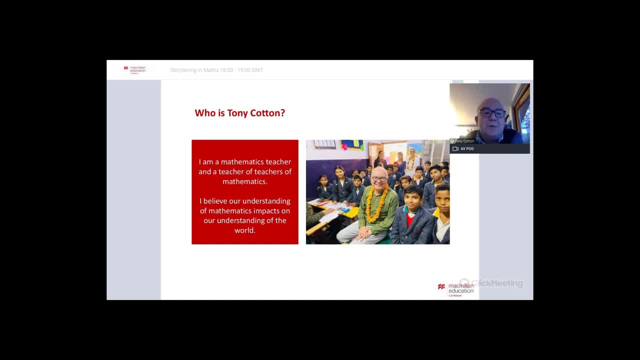 it's a way of actually interacting with many more people than we, than we used to be able to. I also use the phrase: I believe our understanding of mathematics impacts on our understanding of the world, And I think that is why I teach mathematics. I teach math. 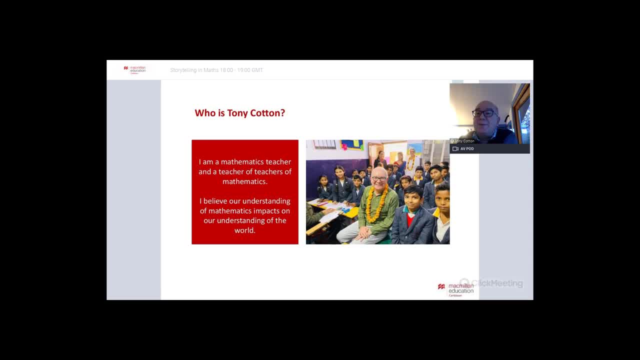 to teachers of mathematics, because i want children to learn mathematics well and i enjoy working with teachers in exploring how, together, we can teach mathematics well in order to develop mathematicians in our- in our- students. you might remember that last time i used an example of of modeling the covid virus as a way of using mathematics to help us understand the world. let 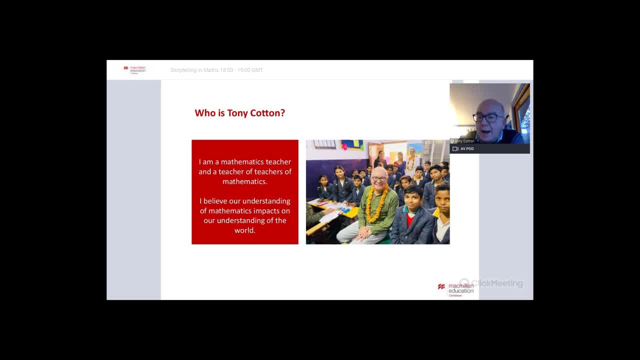 me use a different example this time. i want you to try and estimate how long it would take you to count to 12 million. if you started at one and started counting one, two, three, four, five, six and so on, how long would it take you to count to 18 million out loud? so start thinking. 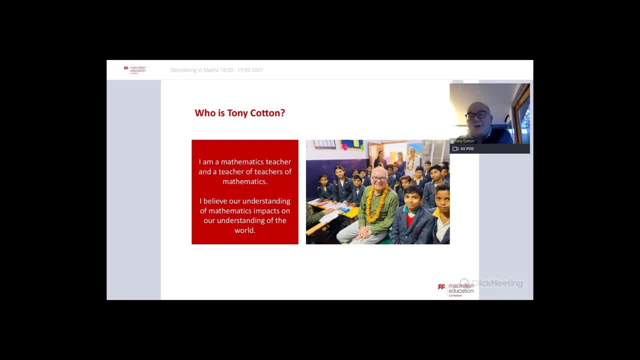 how you might do that and if you can start to calculate that and put some of some of your thoughts in the chat box. that would be really, really helpful. again, as you know the people that joined us last time, we will do mathematics during this webinar. i will ask you to engage in some some 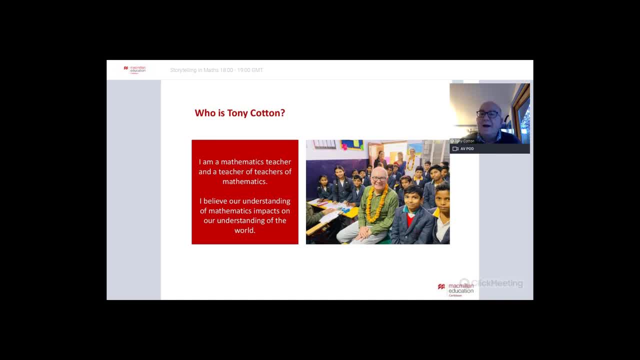 activity. so this is your first activity. how long would it take you to count to 12 million? also, give me a break to have a sip of my coffee and we'll see. we'll see if your- your answers agree with the answers from the people this afternoon. i remain from jamaica. 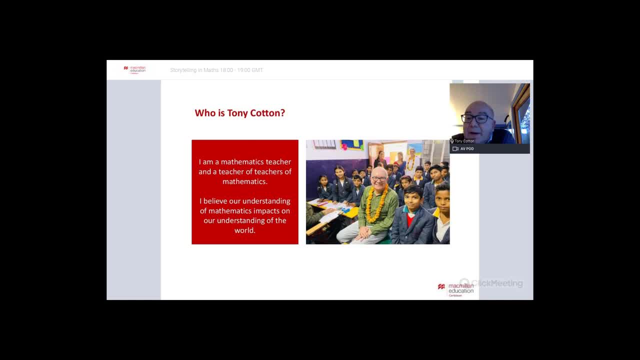 okay, six, 16 million seconds. okay, you work out how many, how how many hours and minutes, or even months and weeks. 16 million seconds is poshy and tracy. and how, how, how long would six million seconds, michelle? how long is 12 million seconds in? is it a week, is it more than a week? is it a month? and tracy i'm thinking of? 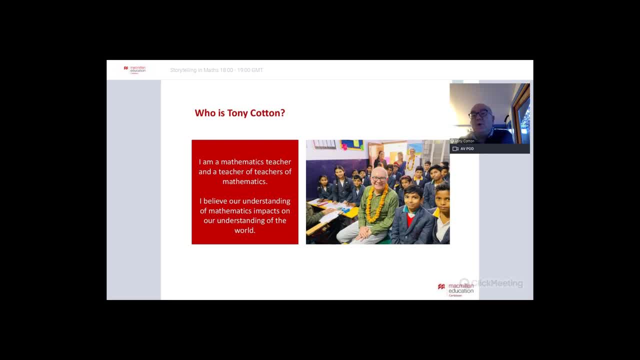 counting two numbers a second. when i get to more than a million, i would be counting. well, let's say, three million four hundred and twenty five thousand one hundred and one. three million four hundred and twenty five thousand one hundred and two. so suddenly it takes me longer. i can say two. i can say two numbers a second. 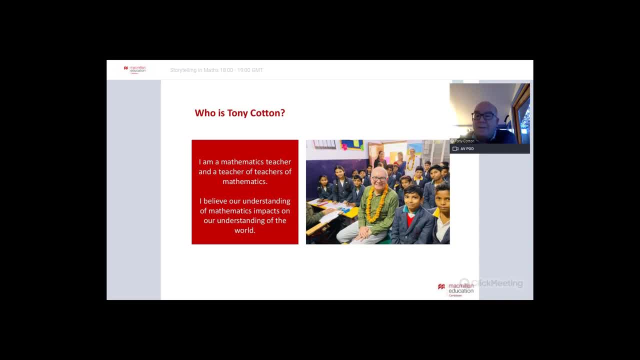 for the smaller numbers, but so it's going to take us longer than 12 million seconds. what do you reckon, michelle, how long is 12 million seconds in? in months and weeks? maybe 12 million is more accurate than six million, because that takes into account. okay, about a month. that's michelle. without that, that would be, i guess, without taking a break. so if you think about taking breaks, if we were actually doing that, we suddenly start to double. double the amount of time. okay, hoshi reckons about 185 days. so that's, that's just over six months. 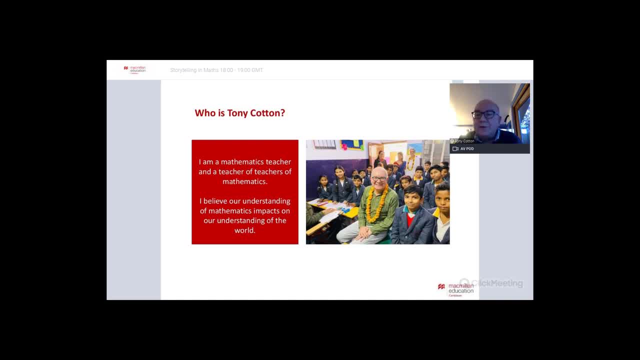 tracy ann thinks five weeks. any other thoughts? i'll wait until this next person's thought comes up, two months from jd. i do apologize if i mispronounce your names. the disadvantage of not being live is you can't correct me. okay. five weeks around the clock. 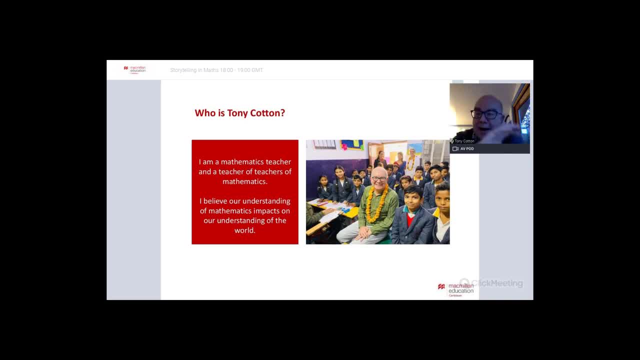 i'm not going to give an answer. um, there are a whole range of answers. i think the answer around six months is probably more realistic in terms of what, what, what people have said this afternoon. um, when i've i've done this task quite often with, with groups of, with groups of people. 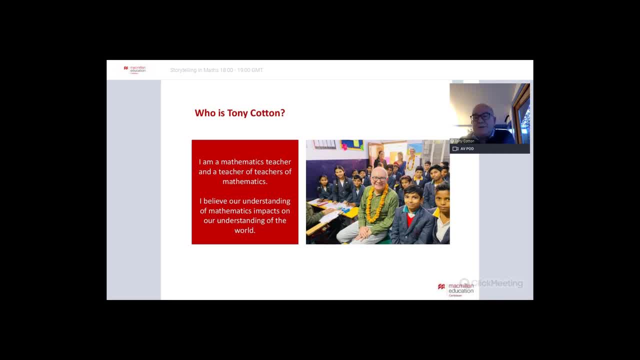 sometimes they time themselves reading out, reading out numbers and taking an average. sometimes they make an estimate in terms of number of seconds and then obviously divide by 60 to find out how many minutes that is. divide by 60 to find out how many hours. 24 for how? 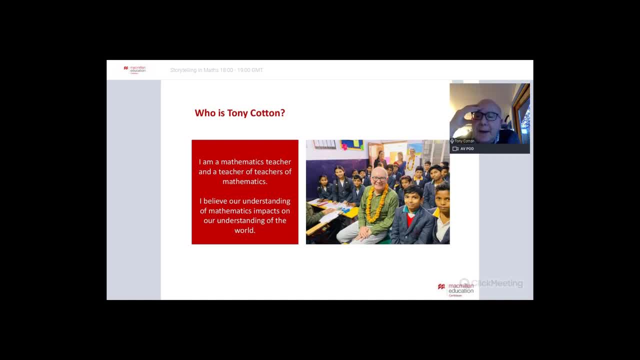 many days, seven for how many weeks and so on, and i think we're probably talking between somewhere between six and six and nine months as a an accurate estimate, and then we also we can agree whether whether that means that we're stopping for break and how long the breaks are um. 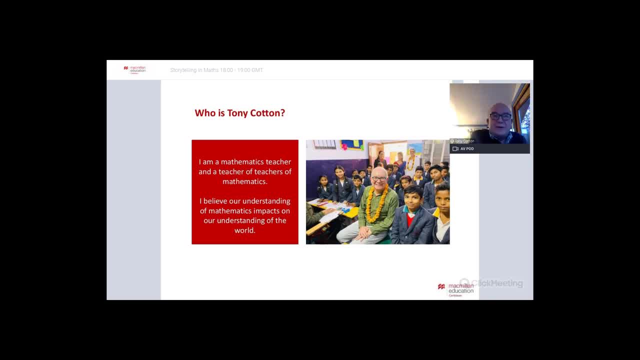 and one of the interesting things, i think is actually having a conversation with students and having a conversation with learners about the fact that there can be different answers and the different answers depend on the constraints that we've, that we've put put on the on on the calculation and on on the problem. now there's a reason that i chose 12 million. 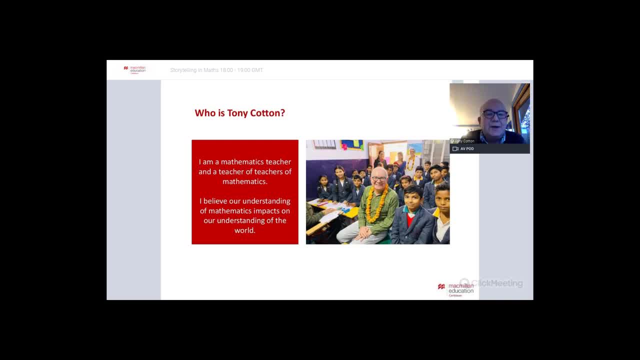 and that reason links back to the. our understanding of theanswexourist, of mathematics, impacts our understanding of the world. 12 million is one estimate for the number of african people displaced from africa during the 400 years of slavery. now, if we say, and suddenly, 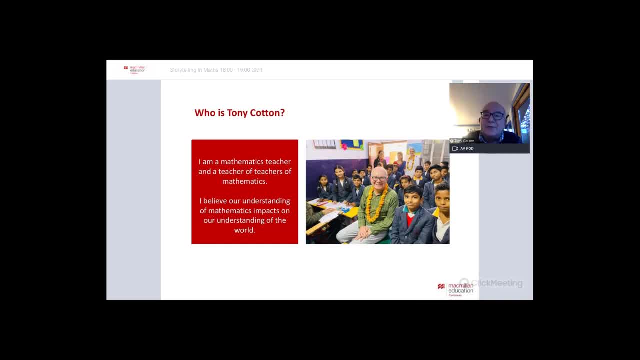 that 12 million takes on a different, a different sense, doesn't earn a different aspect. when i do this activity, live with people, you get a different feeling in the room. there's suddenly a sense of the importance of that number and i think that's an illustration of how suddenly the mathematics 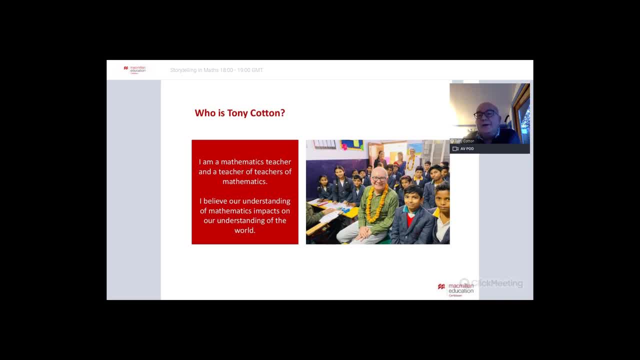 has allowed us to to think about the world in a different way. we understand the evil of slavery at a human level, or we probably can't contemplate the impact that that had on the world and the impact that that had on the world and the impact that that had on the world. 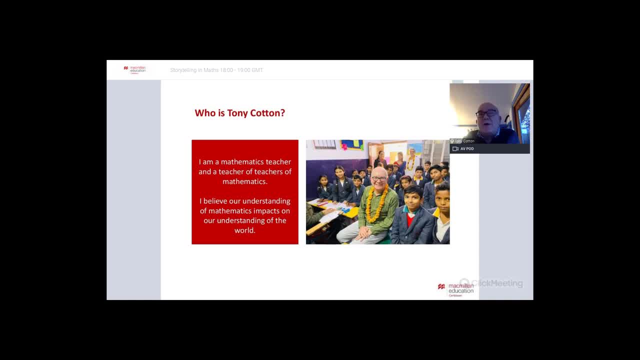 on people without trying to think about big numbers. and 12 million is very difficult to get our heads around in terms of a large number, but if we think it would take us over six months to count all of those people without sleeping, suddenly that number makes some kind of sense. 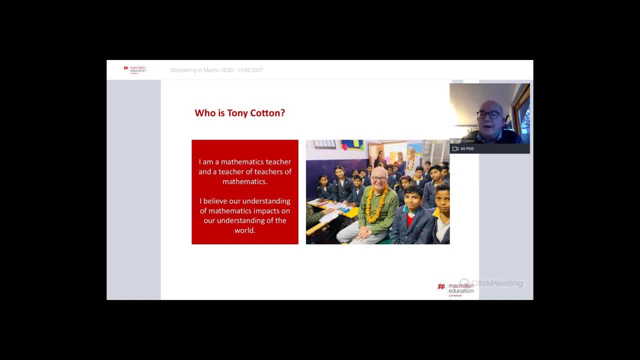 and we get, we get. we can work out how enormous it is. i've i've carried out that activity in europe and we use six million as the number. six million is the number of, of people killed in the, the holocaust in the second, in the second world war and again. 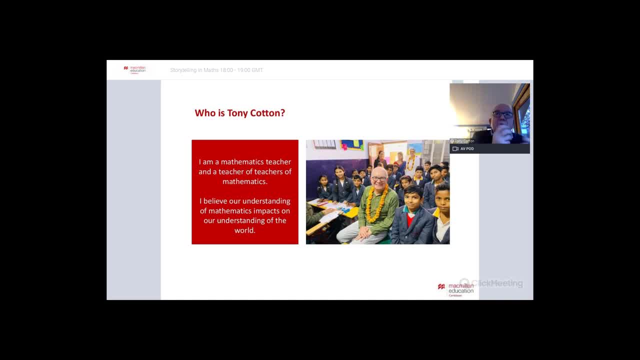 you can feel the, the, the atmosphere in the room change when we kind of understand that number. so that's what i mean about using mathematics to to understand, to understand the world. we can make sense of the world in a different way, and we can make sense of the world in a different way and we 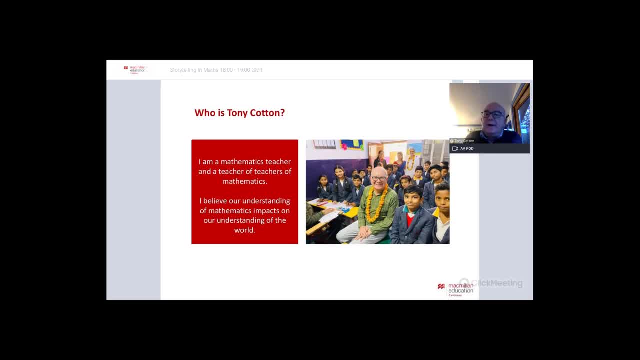 can make sense of the world in a different way, and we can make sense of the world in a different way if we understand the mathematics. now, often we understand the world through stories. we tell stories about the world and we tell stories about ourselves in the world, and i think that's also another way of using mathematics. 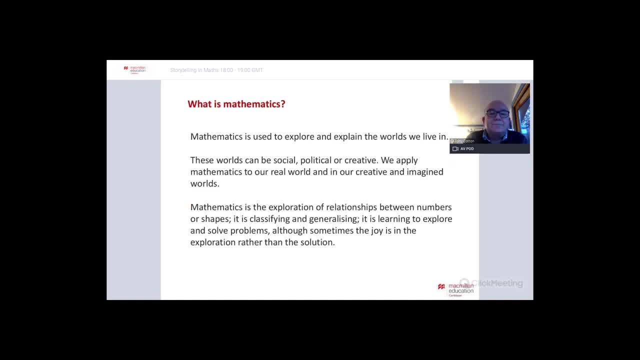 to develop our understanding of the world. the last seminar, the last webinar, was about mathematics in the real world and i used this slide, i used my definition of what mathematics is and i told you it was created from the new zealand curriculum, the uk curriculum, the jamaican curriculum, the belize curriculum, the international 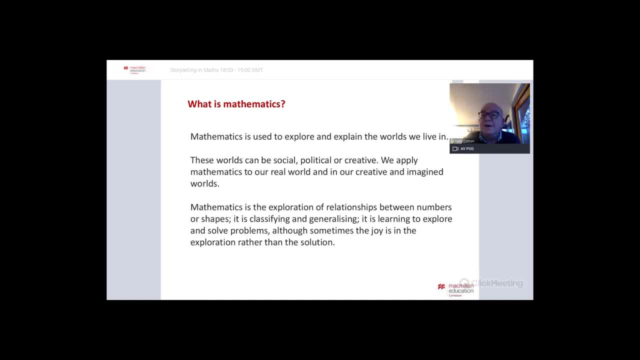 baccalaureate curriculum, trying to pull them all together to get an overview of what mathematics might be. and this is my particular definition and this is the definition that i try and work with in my work. so i think we use mathematics in two ways. we use the: 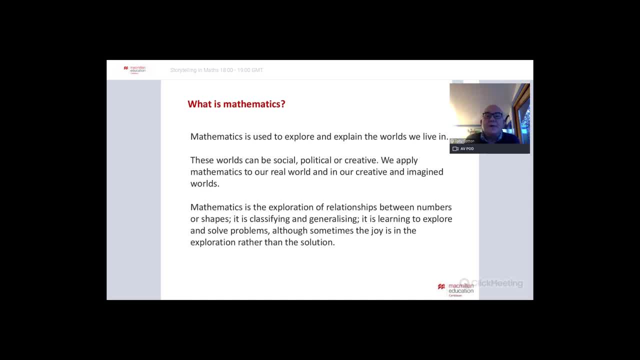 words. we use it to explore the worlds we live in and we use it to explain the worlds we live in, and without mathematics, we can't explore the worlds we live in as effectively and we can't explain the worlds we live in as well. deliberately using the plural for words. 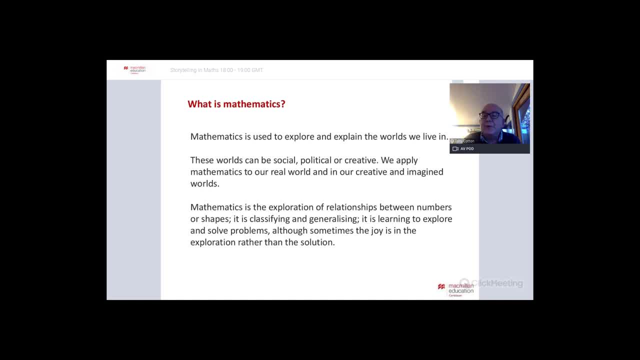 worlds. so the worlds. we have social worlds that we operate in and that can include our work and our teaching. we have political worlds that we live in. what we, what we teach, is decided by our governments. the way that we teach is sometimes decided by our governments. so the political world. 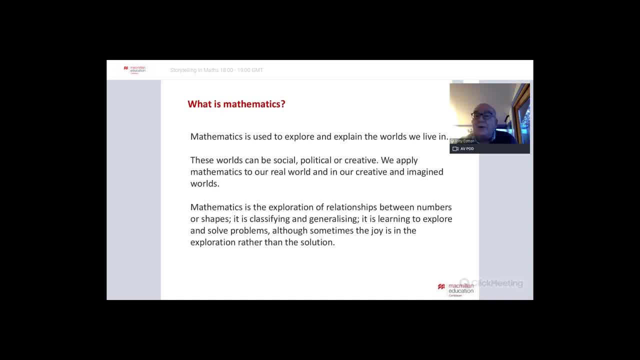 impacts on our, on our social world and on our teaching world and we have a creative world that we live in and those worlds over. those worlds overlap and we explore the world, those worlds, using mathematics and we can explain the worlds using mathematics. And today we are looking at the creative world, And the reason that I think that's useful is that it means we can move away from just seeing mathematics as functional, just seeing mathematics as something that we use in other subjects or that is useful in our everyday lives. 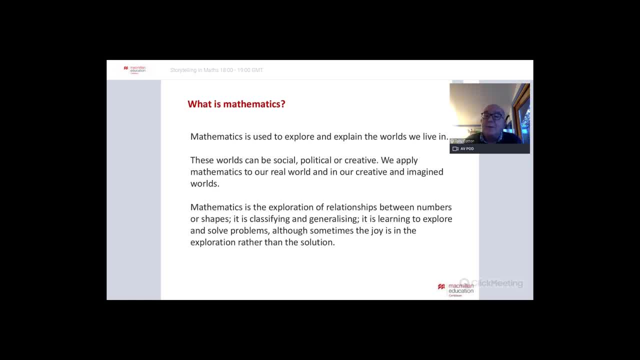 Of course that's an important part of mathematics, but mathematics is more than that. Mathematics can be creative and mathematics can be interesting just of itself, And I don't think we should worry too much about that, because sometimes when our learners, when our students, ask us: what's the point of us doing this? I'm never going to use it in real life. 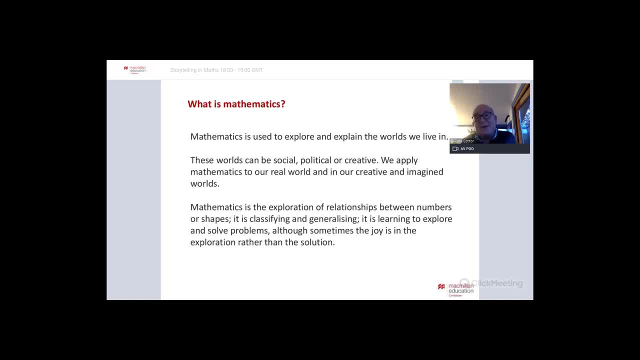 We might say: no, you're not, But it's interesting or it's fascinating or it's creative. And when we're working on storytelling and when we're working on writing, we're not always saying: you will need this for later and later in your life. 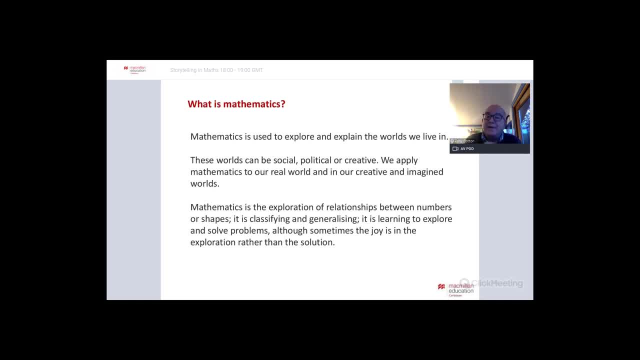 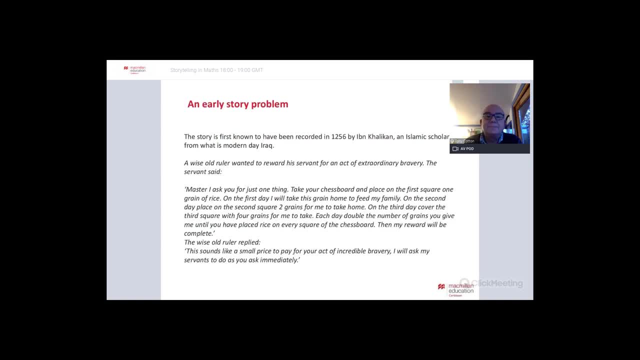 We're saying. this is interesting of itself. So today we're looking partly at mathematics as a creative activity. So let's start with a story problem. One of the interesting things about mathematics and stories is that in the very early days of mathematics, in the very early days of science, often problems were set as stories. 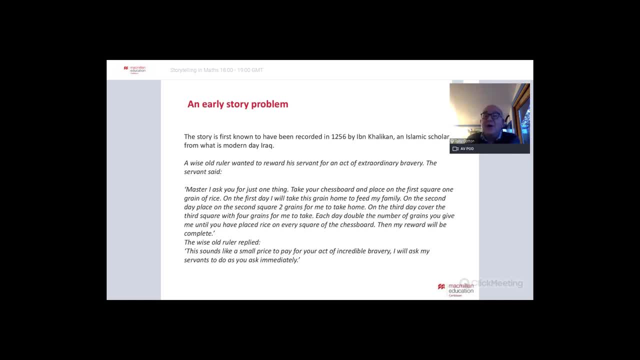 The way that mathematicians would engage each other is by telling a story, And this is an example of one of those stories. And I first came across this four or five years ago, when I was doing quite a lot of work in the Middle East and I was working in Amman, which is just on the Gulf. 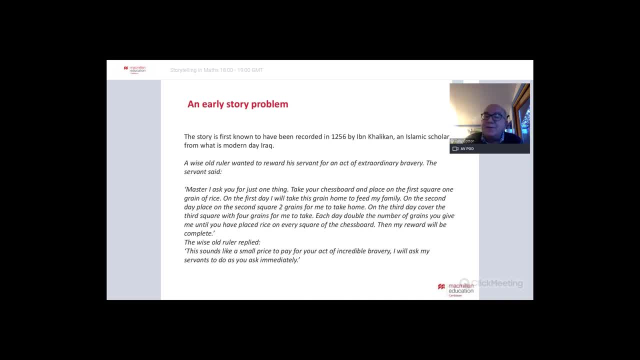 And it's a story from 1256.. So it's an 850 year old story from by Ibn Khaliqan, who was an Islamic scholar in what what's current and what is now Iraq, And I'll just read through this and then we'll we'll think about it. 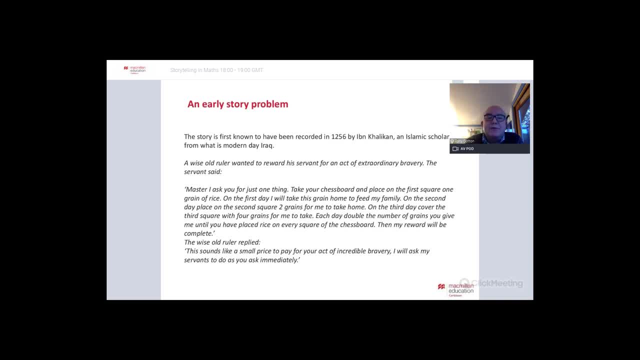 A wise old ruler wanted to reward his servant for an act of extraordinary bravery. Servant said: Master, I ask you for just one thing: Take your chessboard- same as a checkerboard, and play Place on the first square one grain of rice. 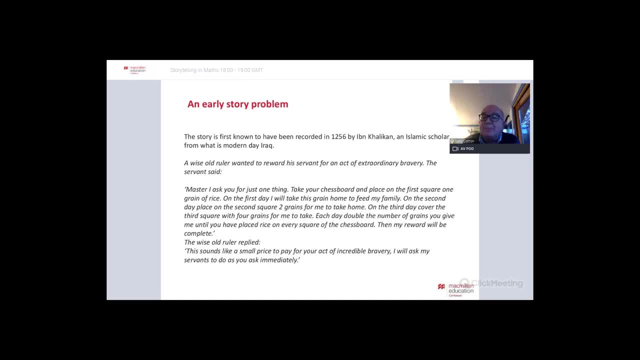 On the first day I will take this grain home to feed my family, So it wasn't going to be much of a meal on the first day. On the second day, place on the second square two grains of rice for me to take home. 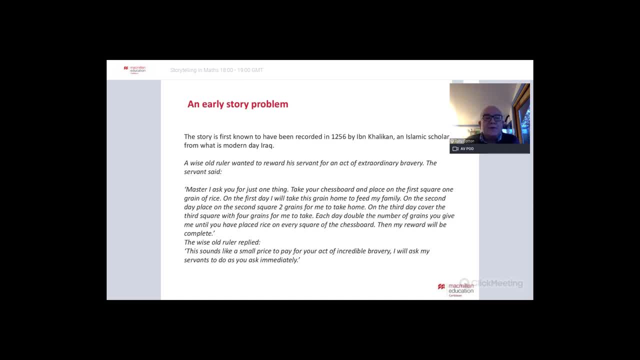 Still not much of a meal. On the third day, cover the third square with four grains of rice. So you can see what's happening. each day He's getting double the number of grains of rice. And that's what he says Each day: double the number of grains you give me until you've placed rice on every square of the chessboard. 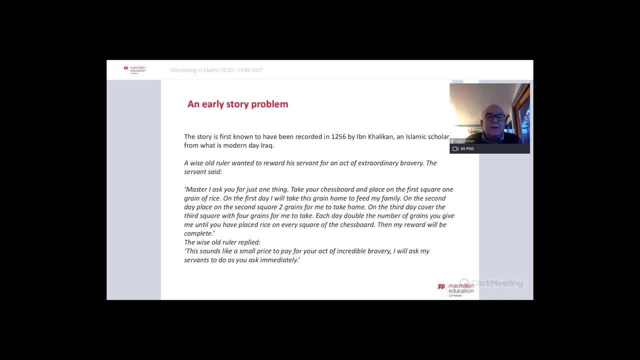 Then my reward will be complete. The wise old ruler replied: this sounds like a small price to pay for your act of incredible bravery. I will ask my servants to do as you ask immediately. So let's work out, Let's think about whether or not it's a. it's a small price to pay. 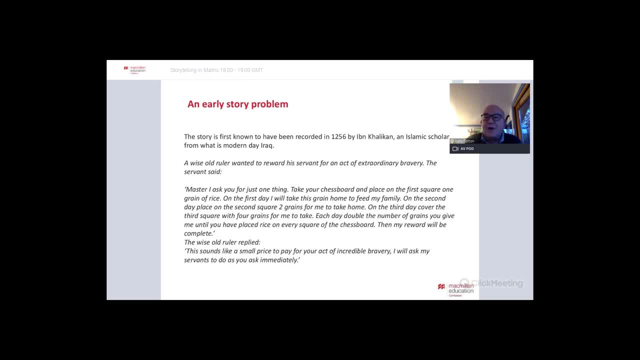 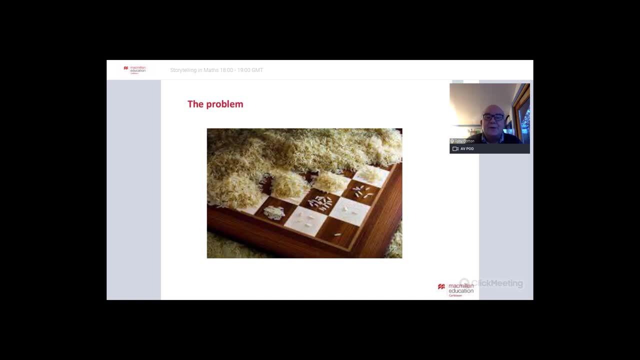 So what we're doing is we're Doubling the number of grains of rice on each consecutive day. So on day one you can see there's one grain of rice on that square. On day two, there are two grains of rice. 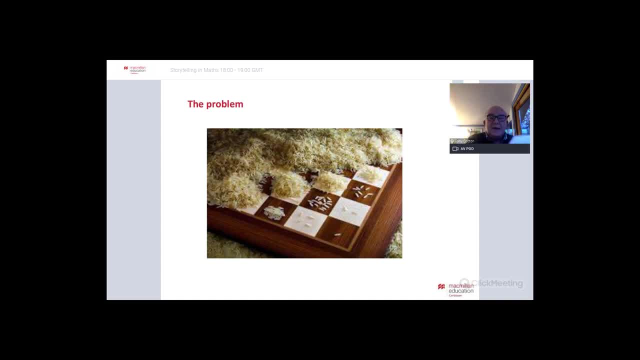 On day three there are four grains of rice. Can you carry on with that doubling and try and calculate how many grains of rice there would be on the 64th square? Now I'll tell you. now it's a lot of rice. 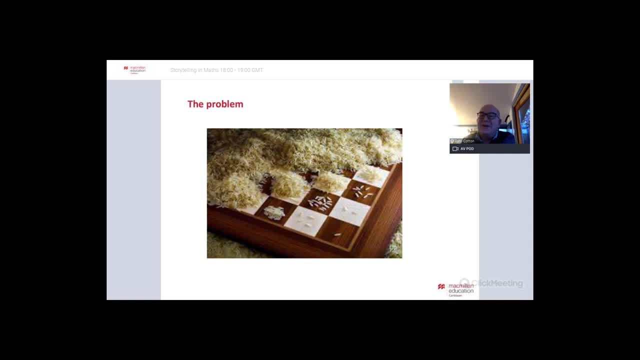 But I'd be interested in you starting to work towards it And again, we'll see how we, how we do compared to this afternoon's, this afternoon's webinar. I'll give you a piece of information in a, in a one pound bag of rice. 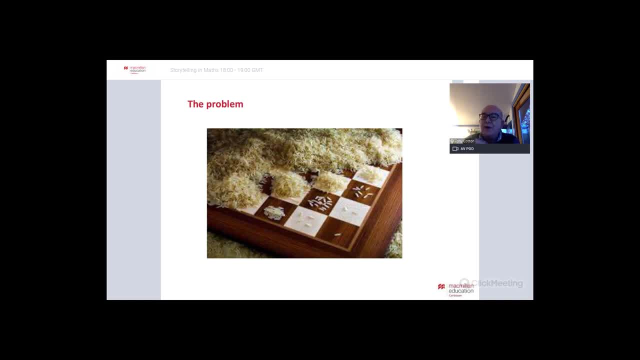 There are twenty five thousand grains. So one thing you could do- and you will need a calculator, Use your phones or use a calculator- is work out on what day Would he be Taking a bag of rice home, or more than a bag of rice? on which day would what would the? would the brave man be taking home more than twenty five thousand grains? 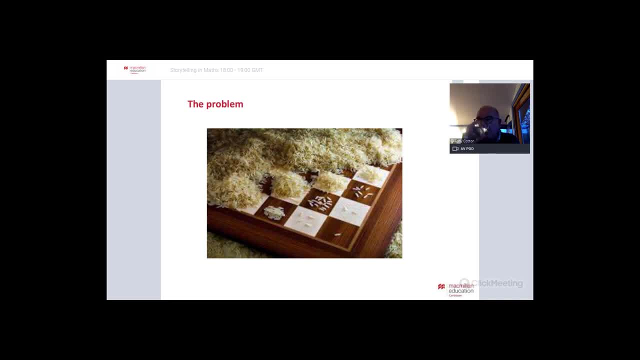 So start doubling and see how it goes. Hi, Alicia and Charlene, in Jamaica, we had- we had a lot of people from Jamaica this afternoon and we're nearly up to two hundred people, which is which is fantastic. So we've got two hundred people doubling and let's let's see where we get to. 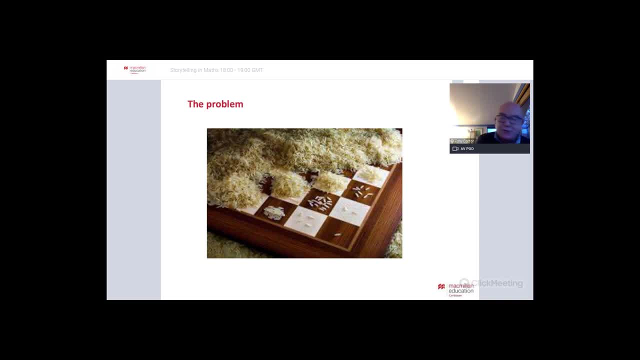 So see how how many times you have to double. to get to twenty five thousand is your first test. So two million, two million and forty eight thousand, which square is that? that's not quite the 64th square. I wonder which square that was. 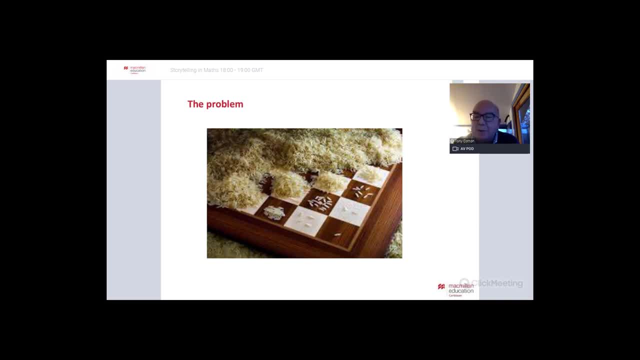 Thanks, Douglas. OK, so to explain to people: Two to the power. sixty three means two multiplied by itself. sixty three times. Now, as with, as With the twelve million, that doesn't give us a sense of how much. how much rice to the power. 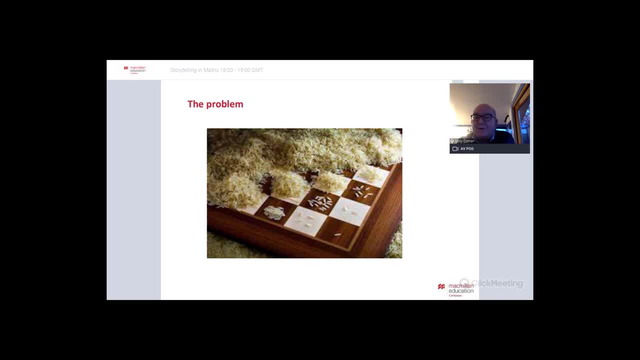 Sixty three is a very, very big number. Can you, can you create a number, Douglas, so that people get a sense of how big that is? Which square do you get? fifteen thousand six hundred and twenty five grains of rice on Nicole? 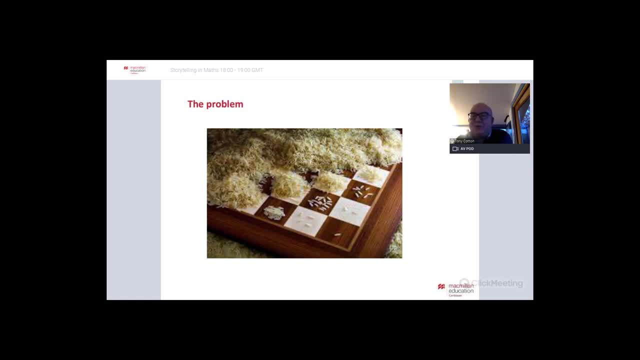 Now it's made small than that. if you double to sixty Four times, you're going to get to more than fifteen thousand. honestly, OK, I'll show you what to the power sixty three or two multiplied by itself Sixty three times looks like. 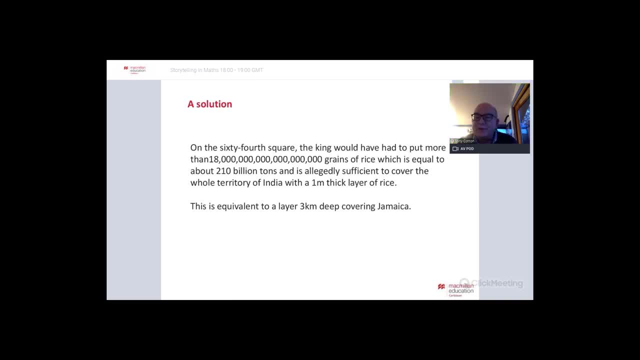 I'll let you think about that while I tell you another- This is a true story this time- And that when I was a small child, I used to double: Thanks, Douglas. So that's Over nine million million million lot of rice is a geometric series because you're- and it's a very early example of a geometric series. 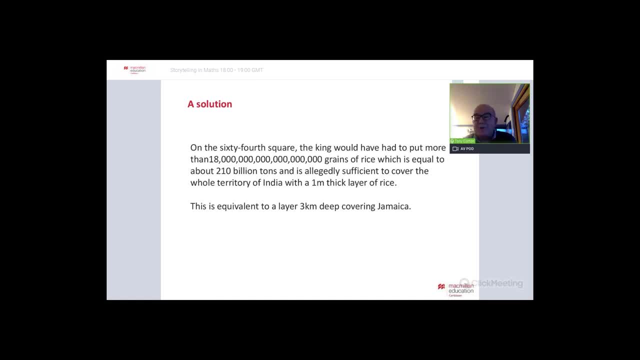 A geometric series is when you multiply by the same number each time. So in this case we're multiplying by two each time, And I was saying that as a small child. I used to. I remember sitting in the back of my car- the car with my mum and dad going to my grandma's, and I would double as far as I could possibly get in my head and which. so I would go- one, two, four, eight, sixteen, thirty two, sixty four hundred and twenty eight, two hundred and fifty six, five hundred and twelve a thousand and twenty four, until until I couldn't do it anymore. 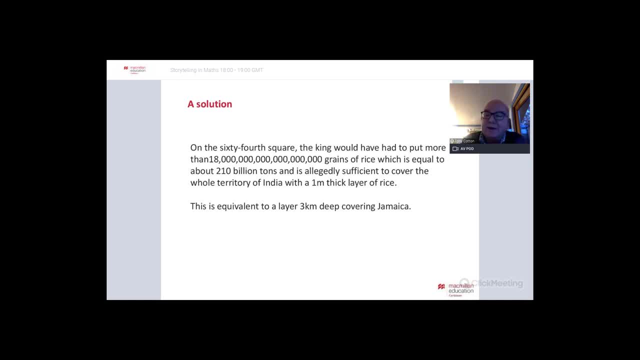 And then I'd write down the answer and see if I could get, see if I get Get further, further next time. So this story problem, this story that was told On the 64th Square, there would be more than 18 million, million, million grains of rice, which I'm apparently is two hundred and ten billion tons of rice. 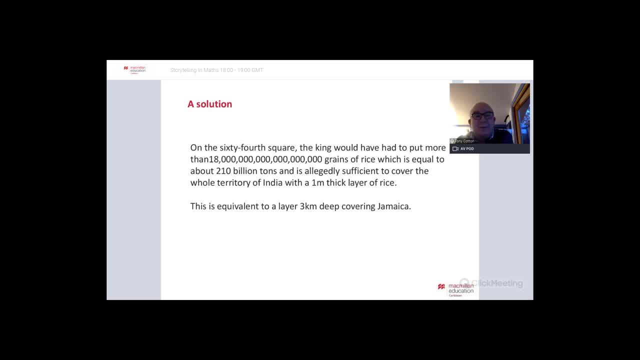 And when I was exploring the problem, when I was teaching in a man, the example I used was That it would cover the whole of India with a one metre thick layer of ice. There are 64 squares Tracy And it's an eight by eight board. 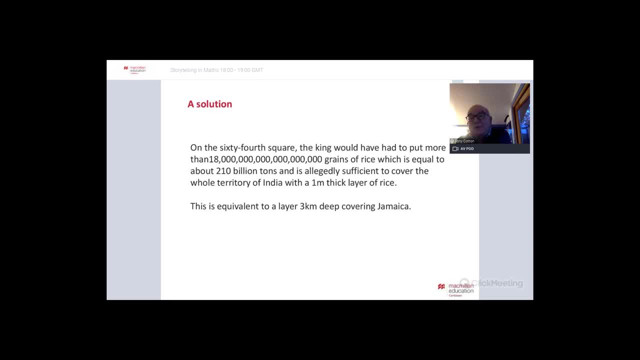 And coming closer to to your homes. That would be the same as having enough rice to cover Jamaica the depth of three kilometres. Now, that's a lot of rice, But it kind of gives us an image of how much of what the how much rice there is. 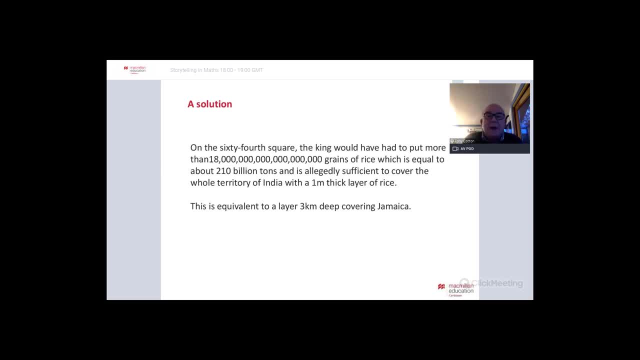 We get a sense of it, don't we? We can suddenly get a sense of it, And then what we could do is we could work with that and say, OK, is that, how long would that rice feed the whole of Jamaica for? 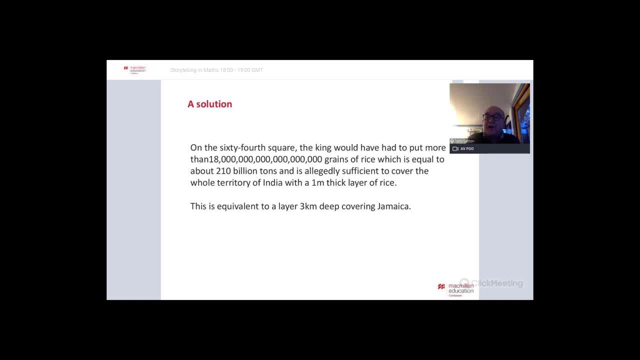 And we could calculate that, we could say: is that enough rice to feed the whole world and for how long could it do that? so we can start to to Work with those big numbers in different ways, But the story has engaged us in doing some mathematics and making, making something interesting. 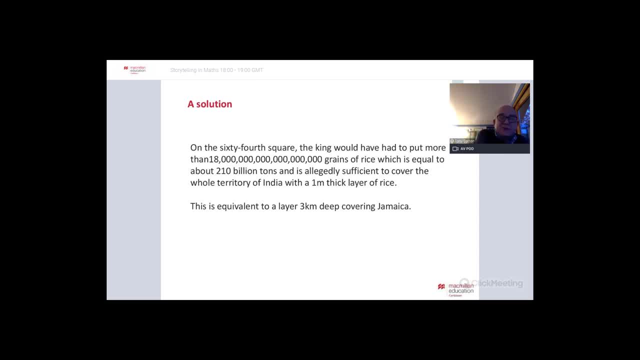 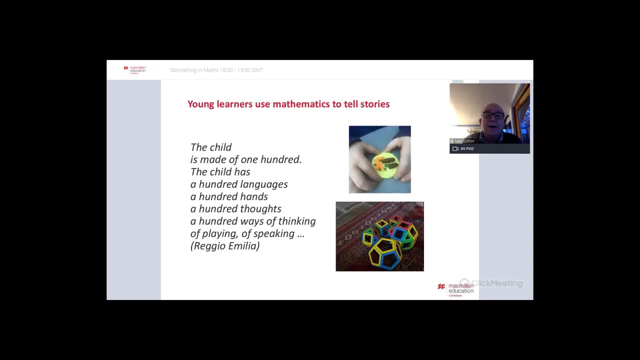 So that's. there is an example that stories and mathematics have been intertwined for at least eight hundred and fifty years, and actually longer than that. Well, well, whatever there's been mathematics, it's been told through stories And again, I used that. I used those images last time because, as I was thinking about this webinar, I was remembering the last webinar about real worlds. 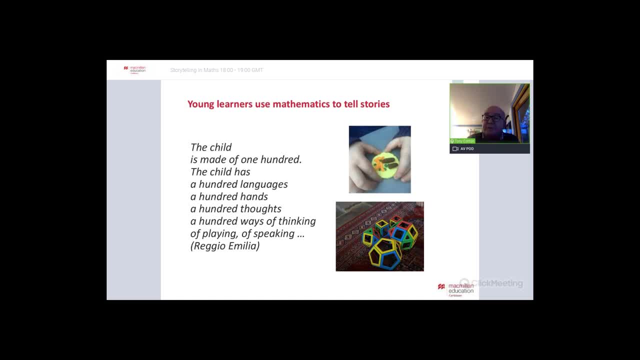 And I remembered using this slide as an example of real worlds. So the top image of this, of the very small model of my, of my tea, of my sausage and carrots and peas, It's made by my take my three year old grandson and the three dimensional 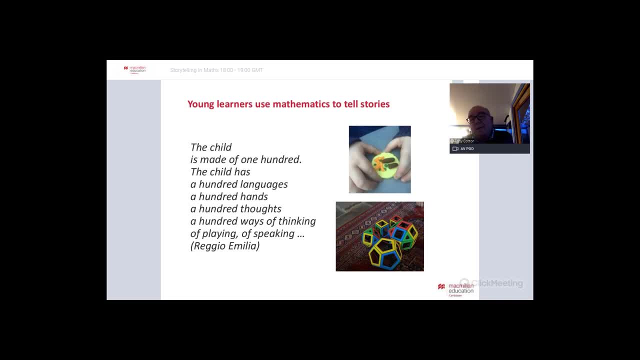 Shapes made out of the magnetic polydrom were being were made by my eight year old grandson And I used the example there of Reggio Emilia and saying that mathematics was one of the languages that children had to explain their worlds and to explore their worlds and to speak about- about their worlds. 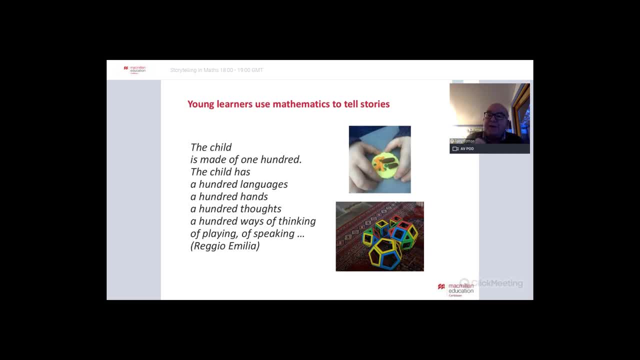 But when I thought about it, both Tate and Felix actually told me stories. they created their own stories about the mathematics that they'd been doing. So Tate was telling me about the cafe that he was working in preparing the food and who was coming into the cafe. 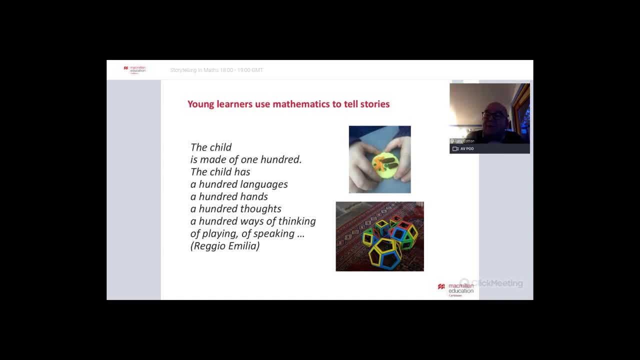 So he he'd done the mathematics in order to create the plates of food. in the context of telling a story, Felix was telling a story. He told me that the largest of those three dimensional shapes was a sports stadium. The next largest of the three dimensional shapes. 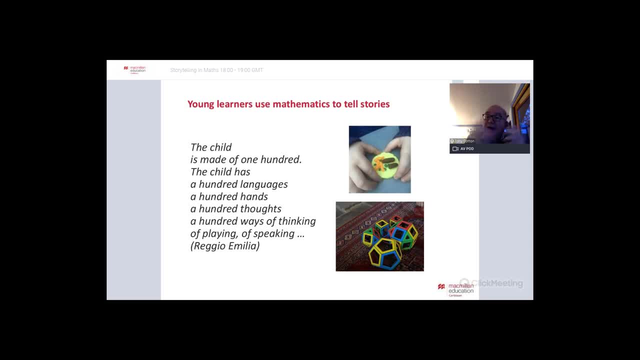 Was a conference center, The next one was a hotel, And he was telling me stories about what was going on in those places. So it seems to come fairly natural to young learners to tell stories using mathematics. If they have developed their mathematical language, if they see the world in a mathematical way, they will tell stories using mathematics and they will interpret stories using mathematics. 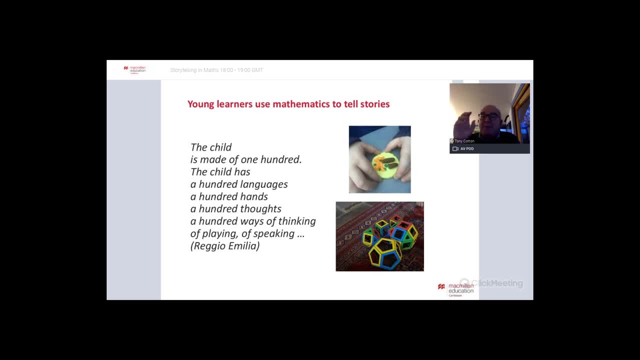 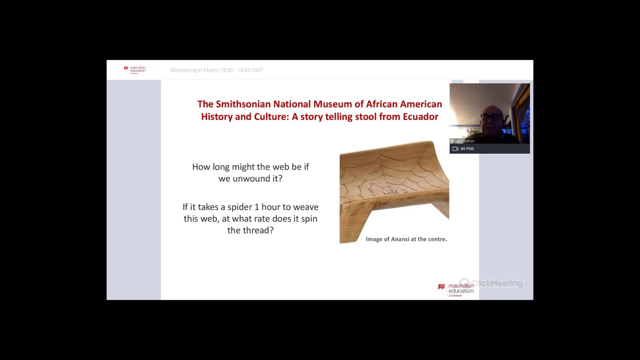 And I think that's kind of what I want to look at- is by They will start to see Mathematics in the stories And then they will start to see mathematics in the world. One of the things that happens to me- I don't know whether it happens to you- is that when I'm, when I'm planning something- 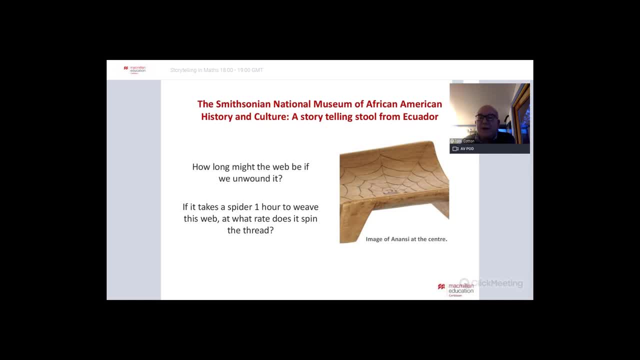 Suddenly, everything I read or everything I look at seems to relate to it. So how do I project that way the thing that I'm planning? So the minute I started planning this webinar on storytelling and stories and mathematics, everything I read seemed to kind of relate to that. 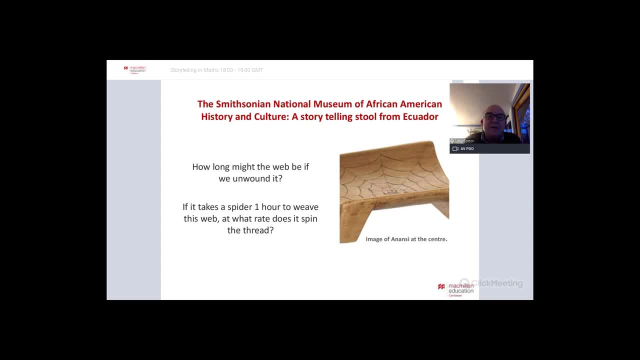 And I was looking at a magazine that I read- It's called the London Review of Books And they had an item. they had an article about a new museum in the States And it's called the Smithsonian National Museum of African American History and Culture And what we have there. 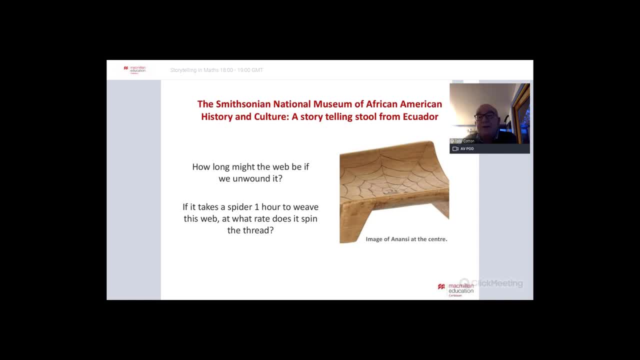 is a storytelling stool that was actually made in Ecuador. Now there's already a fair amount of journeying gone on there, isn't there. So this is Anansi. I'm going to use two Anansi stories later on. So Anansi has traveled from Africa, probably via the Caribbean, to Ecuador. 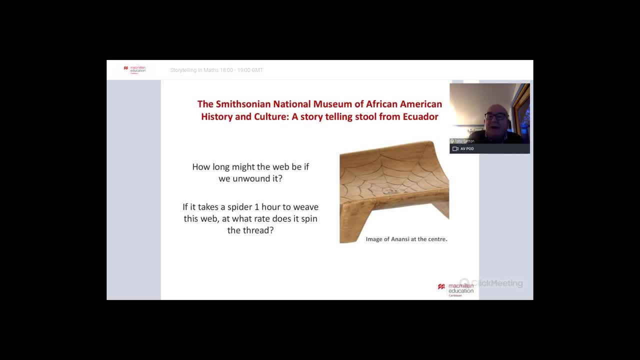 and his stories have traveled with him And here is a storytelling stool with him at the center. Now, I was fascinated by this. I knew I was going to use the Anansi stories as an example of storytelling and mathematics. And I knew that because in my early days as a teacher in the 1980s, 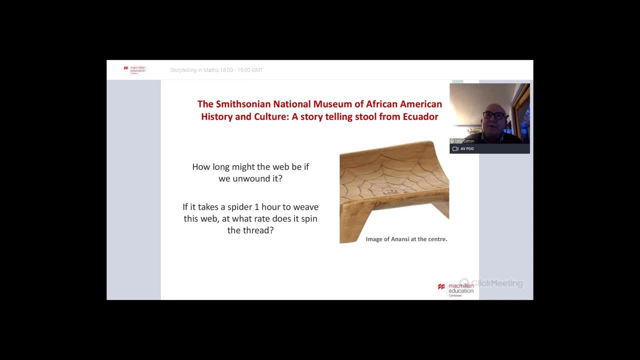 I'm quite old now. I worked at a place called the Center for Multicultural Education and that was in in Leicester, in the Midlands of England, And what we were doing was exploring ways that we could draw on the really rich heritage of all of the kids who come from all. 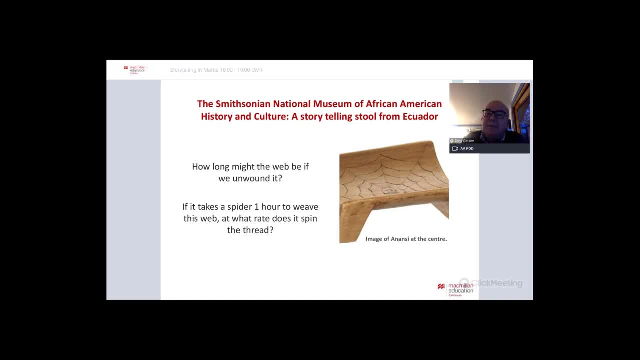 around the world to live in Leicester, and how we could make sure that what we were doing was celebrating all of our, all of our heritages, and drawing on that, And the Anansi stories were one way of one way of one way of doing that. Now there's even mathematics in the middle of the book. 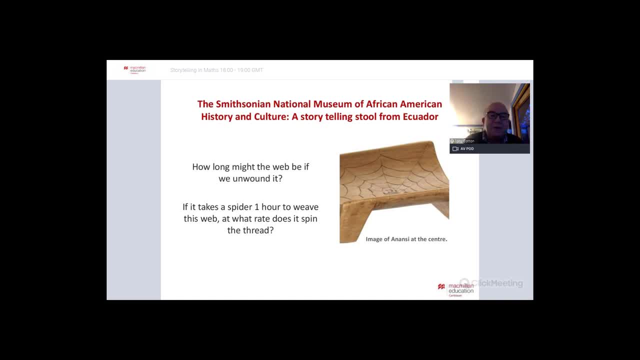 this in this, in this, in this storytelling stool which i'm going to ask you to to think about- and this is an activity that i did do with with felix and tate- so that stool is big enough for one person to sit on. so i think you can get a sense of the dimensions of the stool: how, how long and 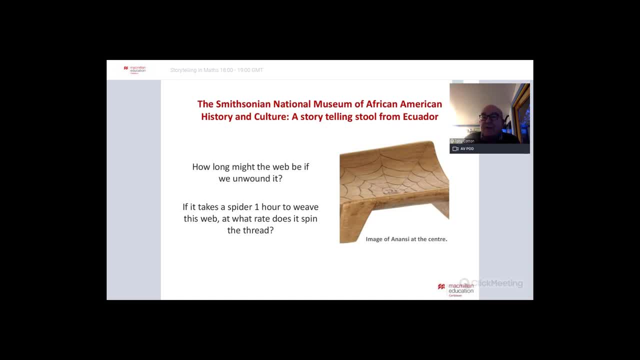 how wide the stool is. if you get a sense of how big the stool is, you can start to think about how long the web would be. so i think the web has has got five loops, if you like, in the spiral as it spirals out. so start to think: how long might that web be then, which is the question i asked, felix. 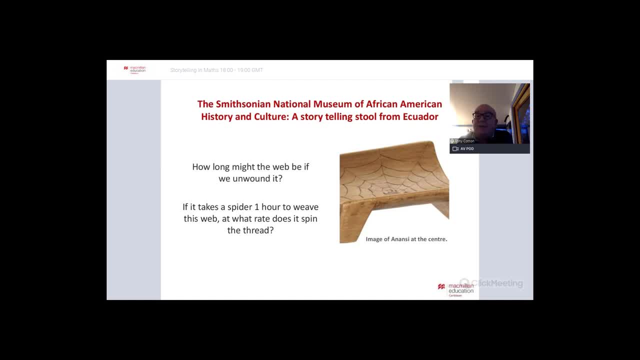 and tate, and then we looked up how long it takes a spider to weave a web and apparently, um, the search engine told me that a spider takes about an hour to weave a web, which seems very quick to me, i. so if a spider took an hour to weave that web, if a nancy took an hour to weave that web, what rate? 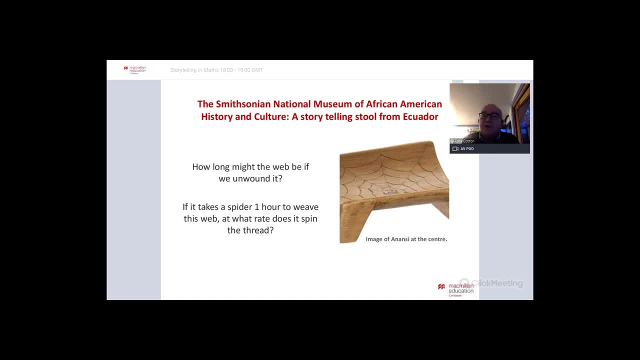 would it be spinning spinning thread? so let's just spend a couple of minutes thinking about that. how long do you estimate that web? is that an answer has worked as weaved? and if, when you work out how long it might be, at what rate do you think the web was spun? 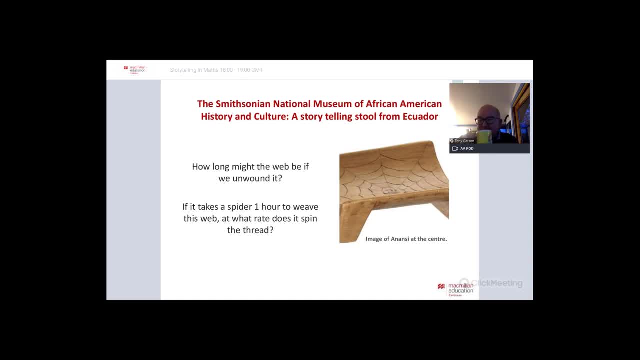 it's always nice to see some someone is someone is typing message come up. what's particularly nice about these seminars is that tomorrow i'm actually going to go over to manchester in the uk and i'll be with felix and tate and i will tell them that i've been sharing. 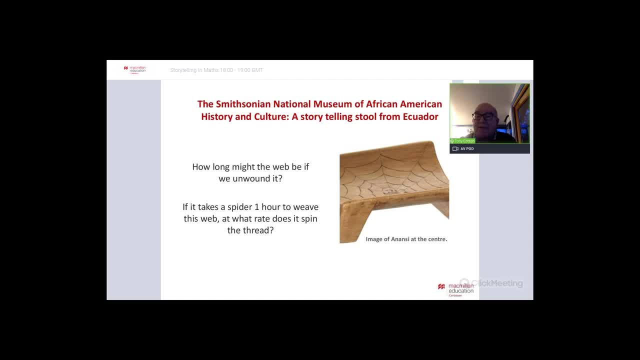 the mathematics that we were doing last week with people in the caribbean, and what i will do is take all of the different places that you're from and we'll look at the world map that we've got and we'll be discovering where you all are. that's how you'd work out, tracy, and can you actually? 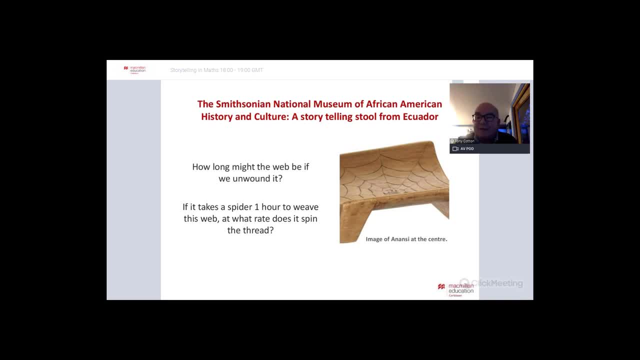 work it out. how long do you think the web is tracy, and thanks ever so much. you're being one of the really good people about joining in, so thanks for thanks for your contributions already. can you do you think you can estimate how long that, how long that web is? 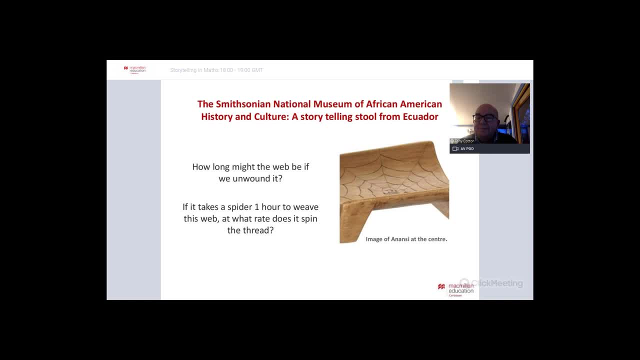 i'm still interested in how long, how long you think the web is, nicole and tracy, and what do you reckon? okay, kena reckons 300 centimeters, three meters. anybody else got any any estimates for the length of the web? and this is another example of an activity which doesn't have an exact right answer. 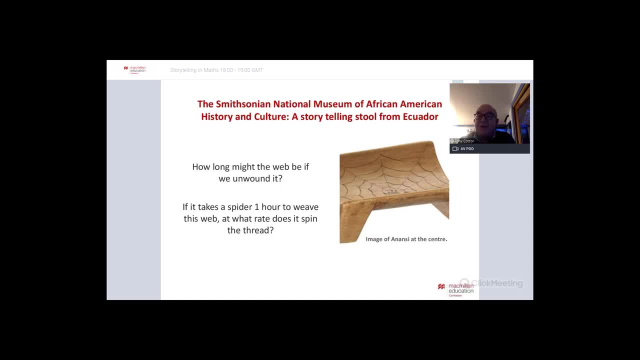 but by working on it together we can. we can get a range of answers and then see which one we think is the is the most reasonable, great thanks. so pedro thinks five meters, jd think thinks one meter. and of course these are all answers because it depends what we've, what we've assumed, the, the dimensions of the stool are. 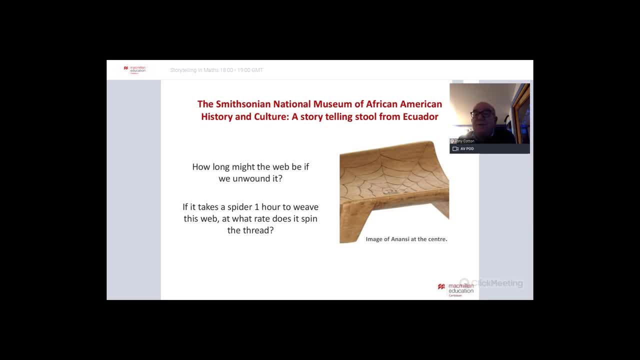 i hope, by the end of this webinar, what you will have is lots of activities you can do with your, the children in your, in your classrooms, what i- that's for you to work out, tracy, and what the dimension of the stool is, and what we- what we did was that we, we looked at this picture and then 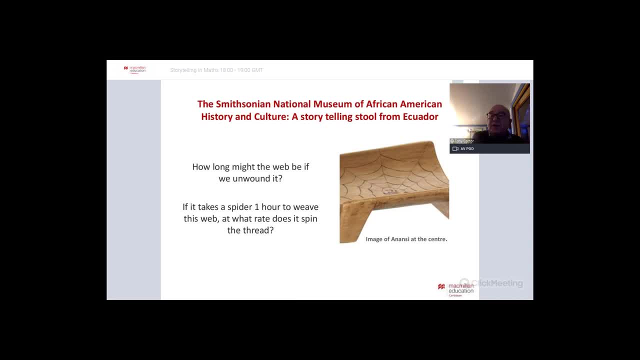 we drew how big the stool would be- it could be as big as an ounce of a stool that we have at home- drew around the top and then we could draw the web on the stool and then we could measure it with a piece of string. so we went through the 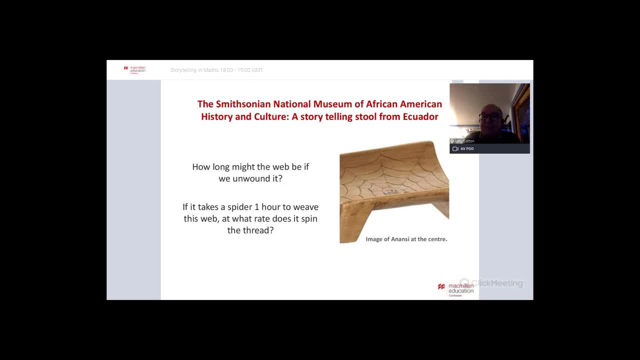 activity that you've just been doing of estimating, and i think that's a really important first step. and then we drew it, and then we opened it out, and then what we actually did was that we split it into chunks. we said, if that long piece of string was an hour, 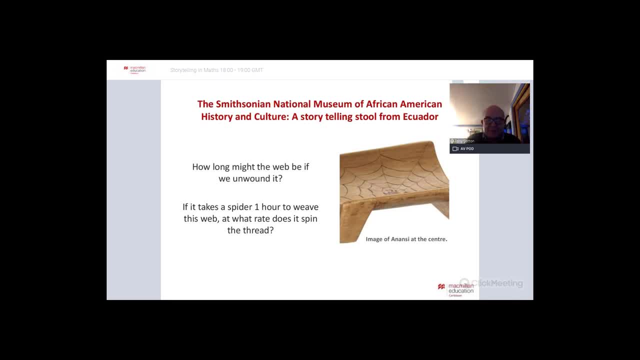 two into chunks of 10 minutes. if we split it into six, they that spider would do that in 10 minutes. and then we can split that into 10, and that's how much the spider would do in one minute. so we could, we could do it all by, by modeling and by manipulatives, and again it's all started to. 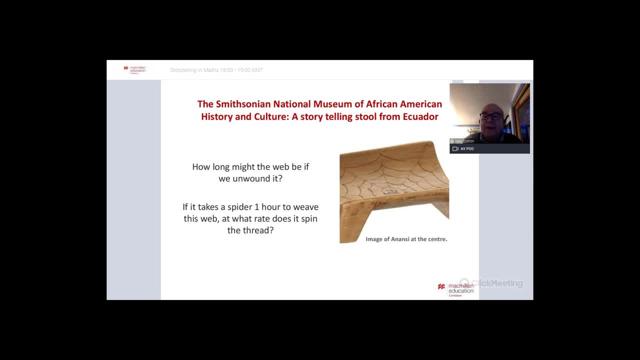 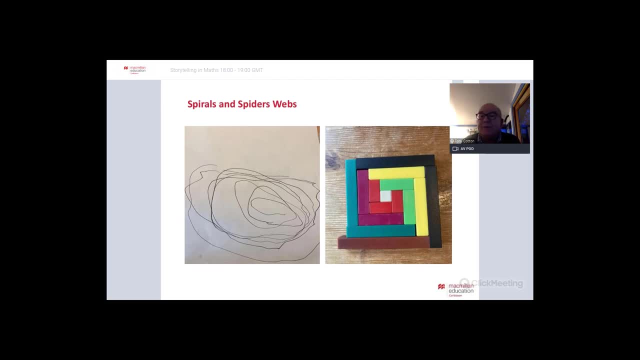 come from story upon me now. as a result of that story, tate h3 went away and started looking for spiders webs. they went back home again. they'd been staying with us when when i worked with them on that activity and the next day on zoom, when i was doing their their maths lessons on zoom. 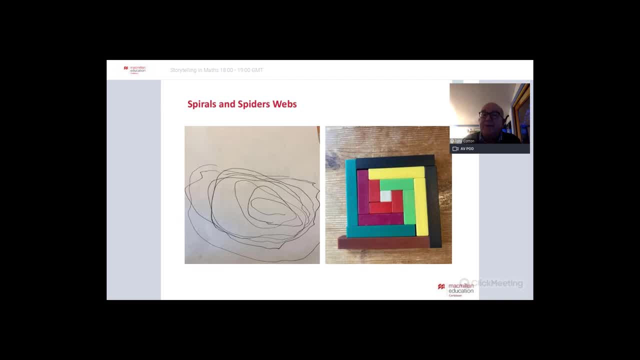 tate said to me: i want to draw you a spiral because spider webs are spiral. and he drew that spiral there for me. um, and he told me lots of stories about spiders. so again the stories were going backwards and forwards. and then i showed him that pattern of cuisine air rods, because we've been doing quite a lot of work with cuisine air. 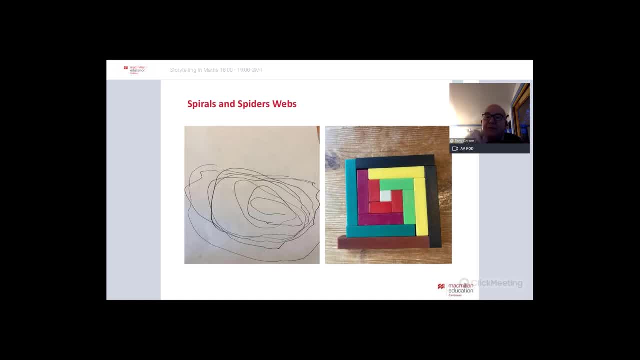 rods, um, and you can see, you can start to see all sorts of patterns in that, in that spiral. so there's a, a white rod in the middle. then that's, there are three red rods which happen to be double the length of the white rod. the green rods are the same length as the red rod and the white rod. 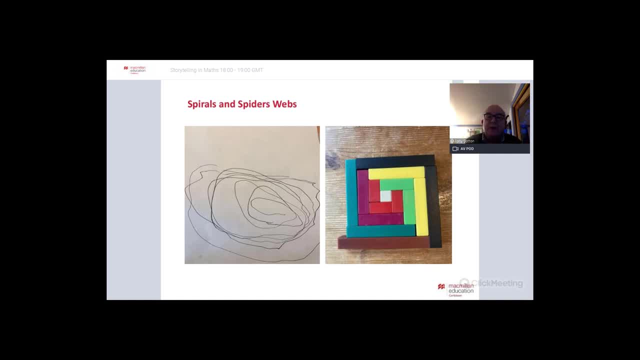 added together and you'll see. then we've got to get two green, two purple, two yellow, two, two dark green. so there are a number of patterns being involved and we were talking about that, um, and tate said that's not a spiral, it's not curly enough. 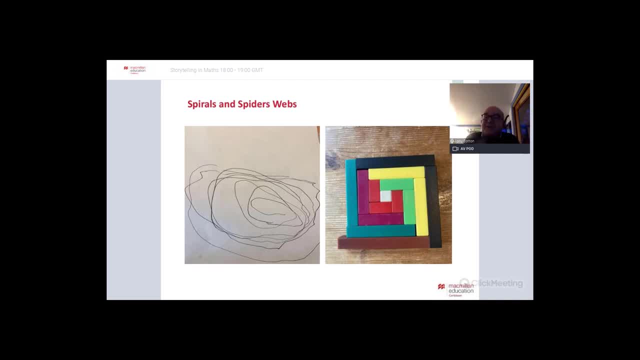 so we started to talk about whether spirals had to be cut, so you can see where there was all sorts of mathematics coming just from thinking about the image of that, of that stool, and you'll find that that happens when you use a story as a starting point. it'll go off in all sorts. 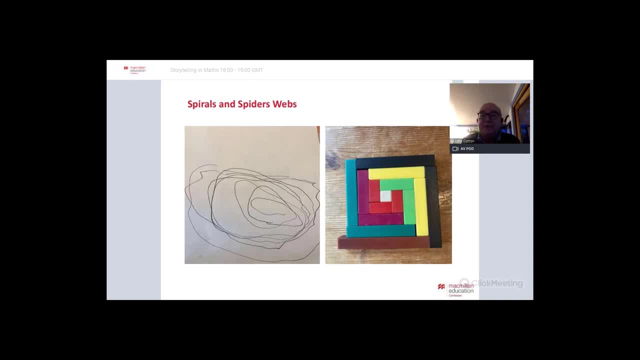 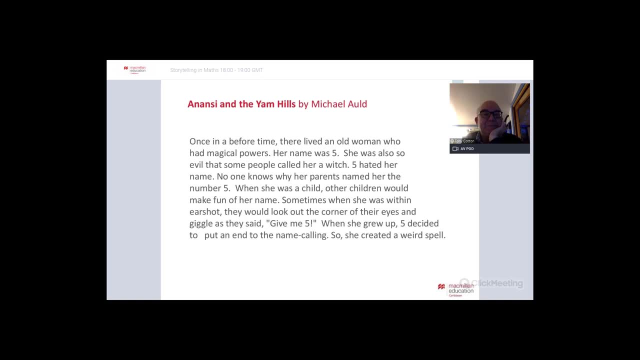 of directions and your own mind will go off in different sorts of directions. you'll think of different ways that you can use it. so let's think about anansi. so this is a version of anansi on the yam hills by michael old. i'm not going to read it all because that would take. that would take. 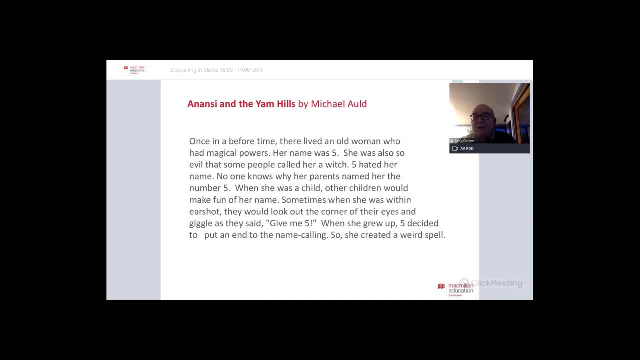 too long, we'll we'll cut through it and then we'll start to think about: um, the mathematics comes out of it and this is where i wish i was with you and i can't read it all, but this is for you to really read what should be happening. is that one? 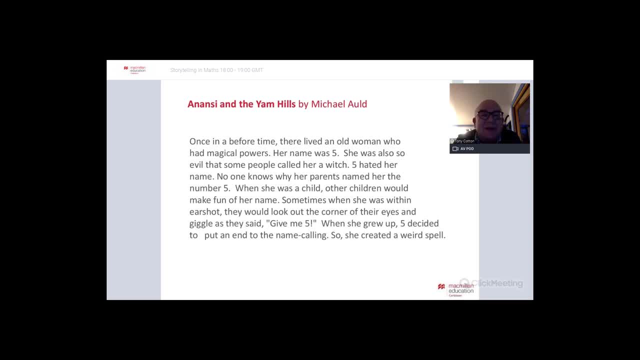 of you should be, should be reading this story, um, rather than somebody in an english accent. anyway, here we go. anansi, on the yam hills, once in a before time, there lived an old woman who had magical powers. her name was five. she was also so evil that some people called her a witch. 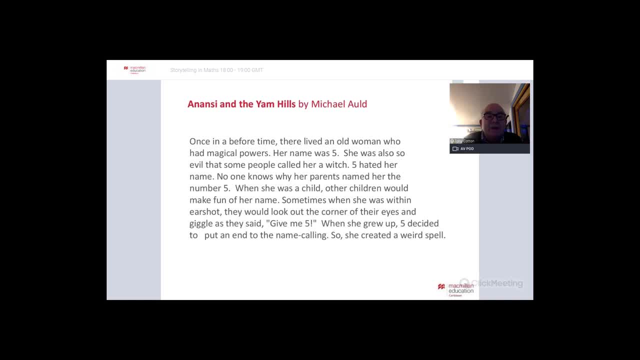 five hated her name. no one knows why her parents named her When she was a child. other children would make fun of her name. Sometimes, when she was within earshot, they would look out the corner of their eyes and giggle. as they say: give me five. 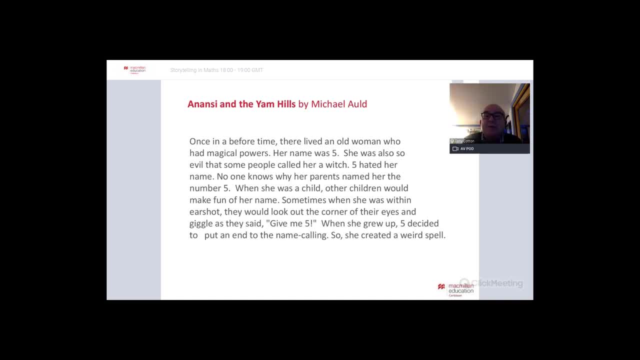 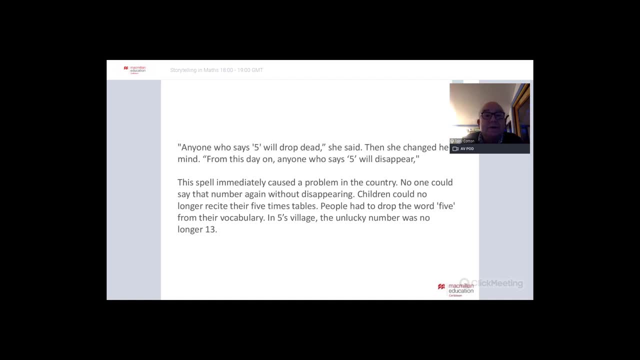 When she grew up, five decided to put an end to the name calling. So she created a weird spell: Anyone who says five will drop dead, she said. Then she changed her mind. No, from this day on, anyone who says five will disappear. 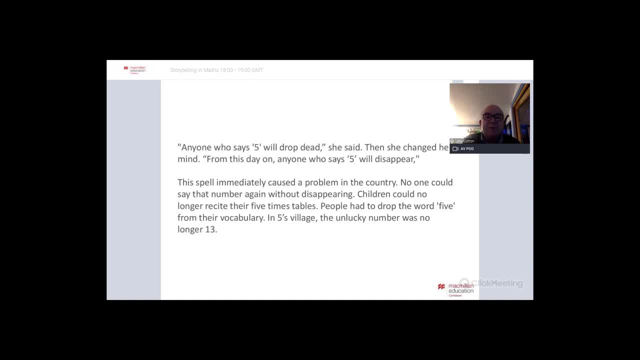 The spell immediately caused a problem in the country. No one could say the number again without disappearing. Children could no longer recite their five times tables. People had to drop the word five from their vocabulary. In Five's village the unlucky number was no longer 13.. 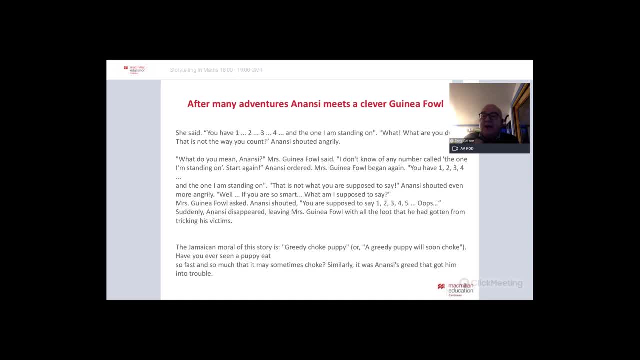 So, Anansi, well, you know the story. Anansi finds out and he starts stealing things from people because he'll stop them on the street And he'll say How many bunches of bananas have you got? And they'll say one, two, three, four, five. 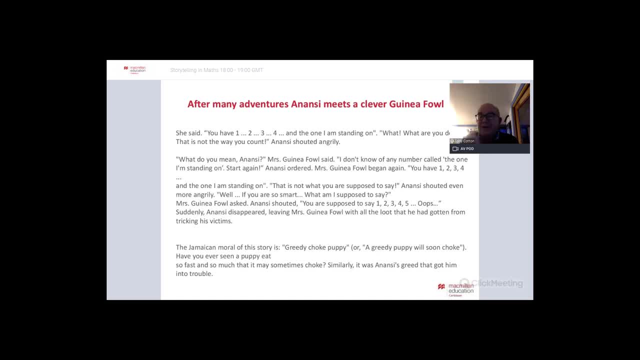 And when they say five, they disappear And Anansi gets all the bananas, and so on. How many coconuts have you got? One, two, three, four, five, And they disappear and Anansi gets all the coconuts. 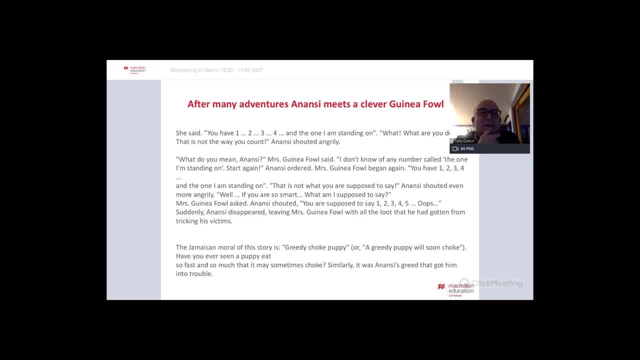 Anyway, eventually, Anansi meets a clever guinea fowl, meets his match. Guinea fowl said: you have one, two, three, four And the one I'm standing on What? What are you doing? That's not the way you count. 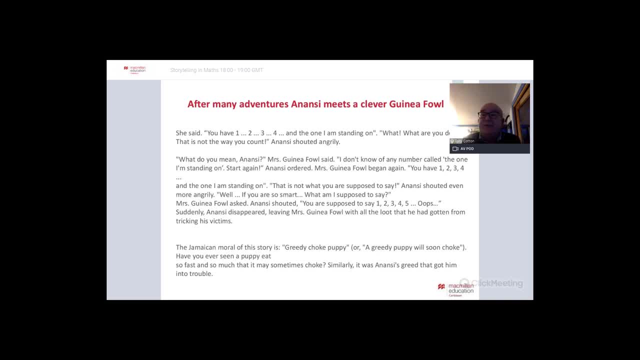 Anansi shouted angrily: What do you mean, Anansi? Mrs Guinea fowl said: I don't know of any number called the one I'm standing on. Start again, Anansi, ordered. Mrs Guinea fowl began again. You have one, two, three, four. 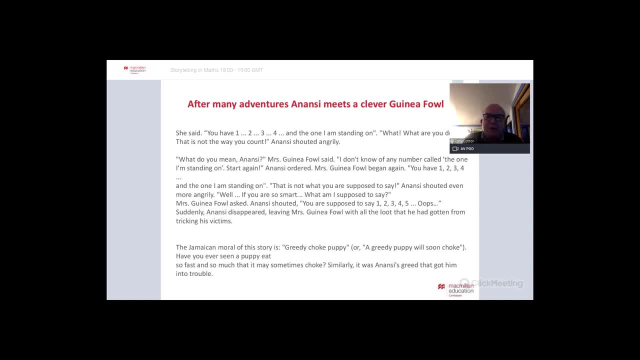 And the one I am standing on. Oh, that's not what you're supposed to say. Anansi shouted even more angrily. Well, If you're so smart, what am I supposed to say, Mrs Guinea fowl asked. Anansi shouted. 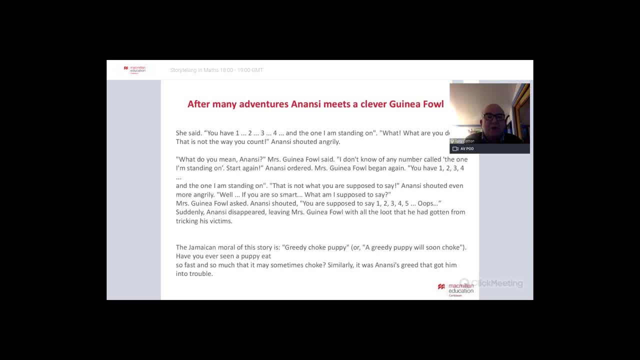 You're supposed to say one, two, three, four, five. Oh, suddenly Anansi disappeared because he said five, leaving Mrs Guinea fowl with all the loot that he'd gotten from tricking his victims, And apparently the Jamaicans. moral of the story is: greedy choke puppy. 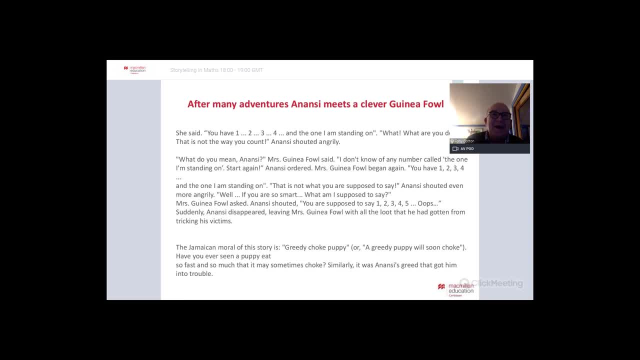 And one of one of the Jamaican colleagues- friends this afternoon told me is it cleave choke puppy, If I remember that correctly, which means greedy. So my Jamaican isn't up to scratch, but I'm learning And I do know that dogs do eat quickly and actually they can get very poorly from eating. 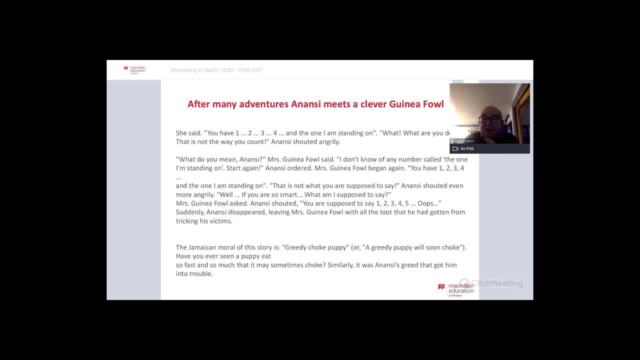 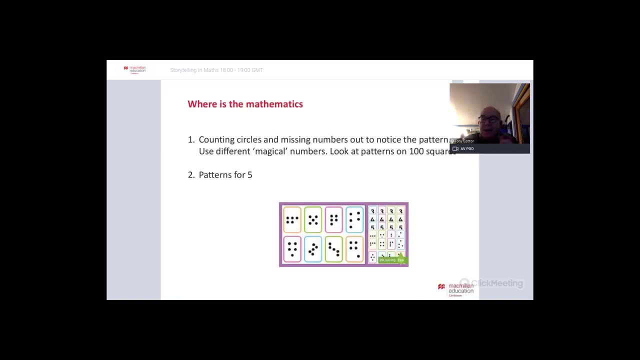 quickly, but it's something, the moral is something about that. Anansi's greed got him into trouble And it seems so obvious. The math is in there. I was fascinated remembering this Anansi story and excited about what I might do with it, because I remember that what I one of the things that I do when I'm counting with children is we quite often sit in a circle and I'll tell them to miss numbers out in a count and clap instead. 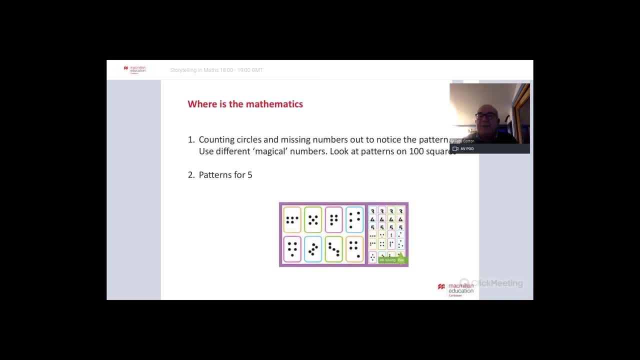 So we might all be sitting in a circle and I'll say that anybody who is an even number doesn't say their number, They just clap. So we go: one, Three, five, seven, So you start to hear the odd numbers. Now you can imagine sitting in a circle and not being allowed to say five, because- because if you say five you disappear. 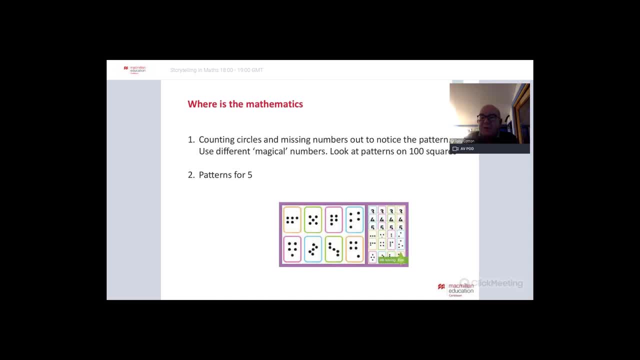 So you clap instead of saying five and you. we could switch it. We can say you're not allowed to say three, or you're not allowed to say four. We can colour in the patterns on a hundred square. So there's any all sorts of things that we could do. 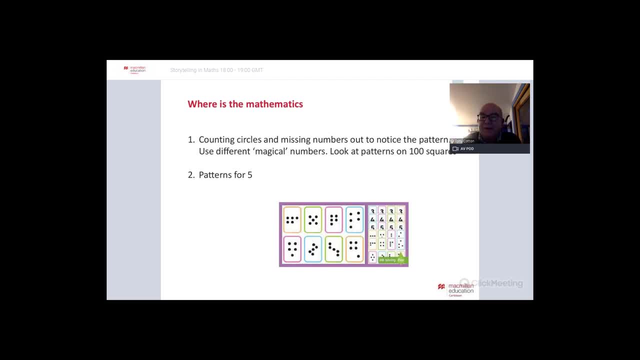 Just taking the not saying five. Five is a starting point. It's a great story, isn't it, Michelle? And then that image. there is an image of different ways of subitizing five. You do it with your three year old Kina. 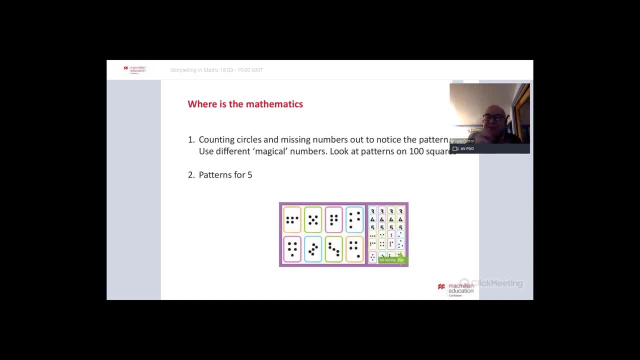 They'll love it. That's great. And so if I'm subitizing- and subitizing means when I can just see a number without having to count, so we can just see all of those patterns of five, can't we, Without having to count. 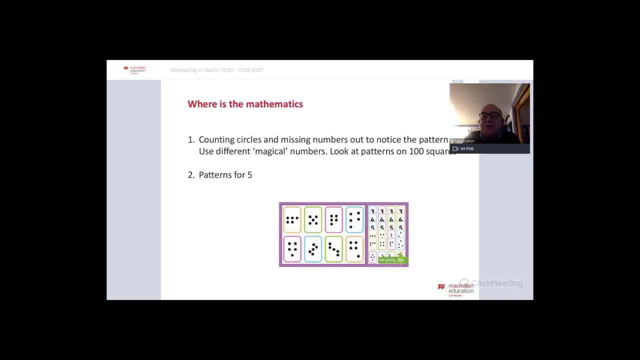 Um, if we think about not, not, not, Not Wanting to say five, we could say two to one instead of five, or we could say three, two instead of five, or we could say two, one, two instead of five, and you can imagine the games that you could play with your, with your children, to avoid saying five. 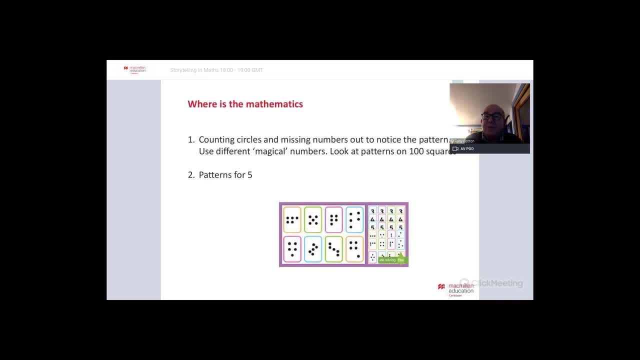 Um, and that gets them to start to see all of the different properties of five. And we can do that with other numbers. So What do people see there? Just quickly put in the chat what you, what you see when you look at that, at that image. 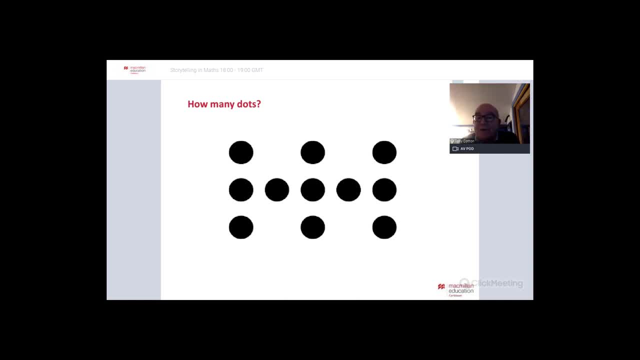 You're not allowed to say 11.. You're not allowed to say 11,, Tracy, and you've just disappeared. Two H's- Fantastic. What do you see in the pattern, Vicky? And there's, there's five in each H, isn't there? 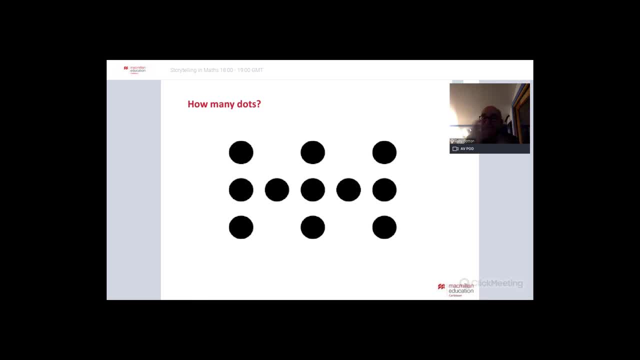 There's seven in each H, but they share There are three. So there's all sorts of different ways that three, three, three, one, one or a five along the middle and ones along the tops and the bottoms. So there's all sorts of different ways that we can start to make dot patterns. 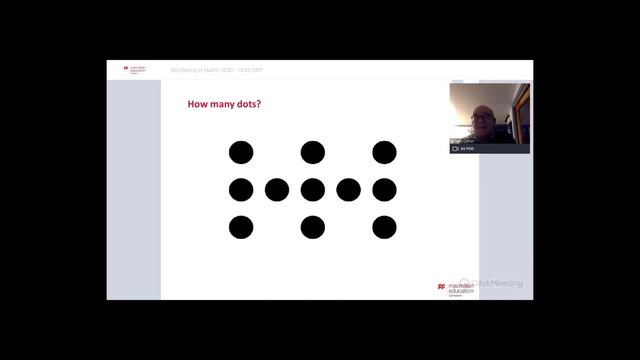 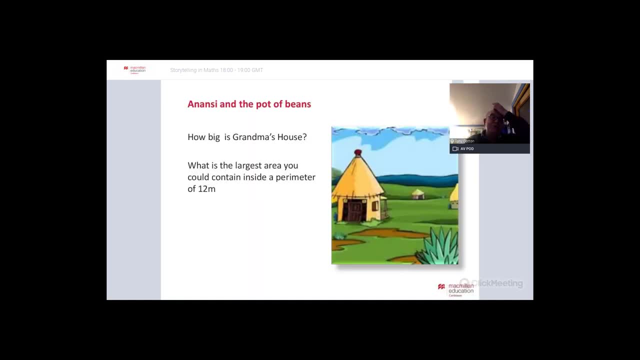 And so one of the things that we could do with the learners is ask them to make dot patterns using the Anansi story as well. Let's just quickly think about another Anansi story and what we could get out of that Anansi story, My my other one that I found was the Anansi and the potter. 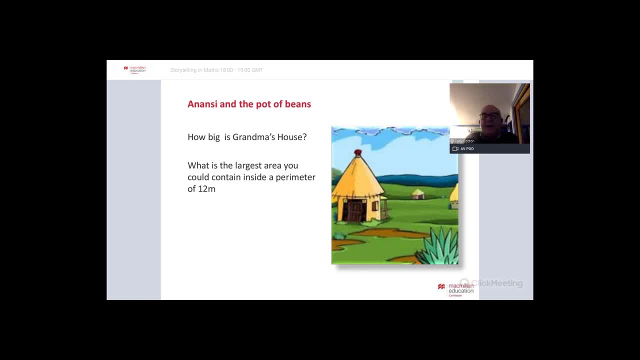 Bean story where Anansi goes to his grandma's house. She puts a load of beans in his hat, asked him to plant all the beans And then she goes. she goes off to market to get the spices, telling Anansi to stir the pot but not to eat any of it. 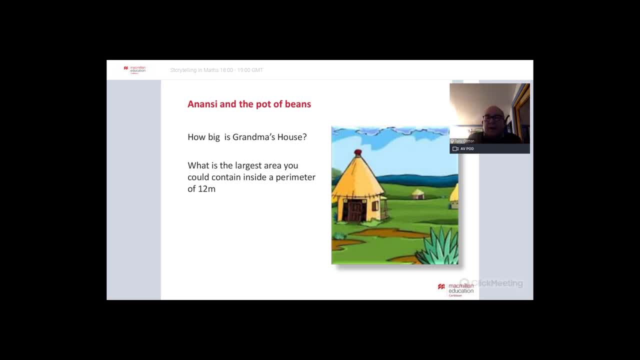 And he's greedy and he eats the beans. And I was reading this story and I was thinking, well, what mathematics can I get out of this story? And straight away I looked at the, the images, and I thought: well, that's interesting because it's a circle. 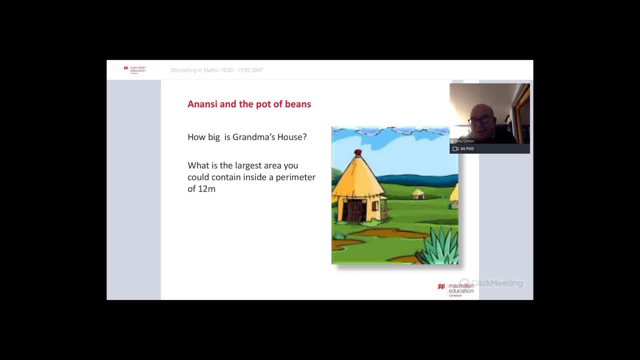 Now, when I when I when I used to fly to places, I was always interesting that when I flew over rural Africa, suddenly buildings moved from rectangular to circular. If you think about igloos, they're circular. Now, the reason those buildings are circular is because a circle can contain the largest area for any given perimeter. 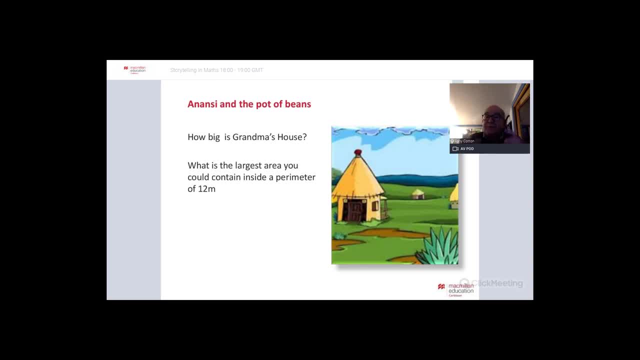 So if we're short of resources, It's best to build a circular floor, because we get the most floor space for a given perimeter. Now, that's an activity that we can explore. That's an activity that we can do thinking about grandma's house. 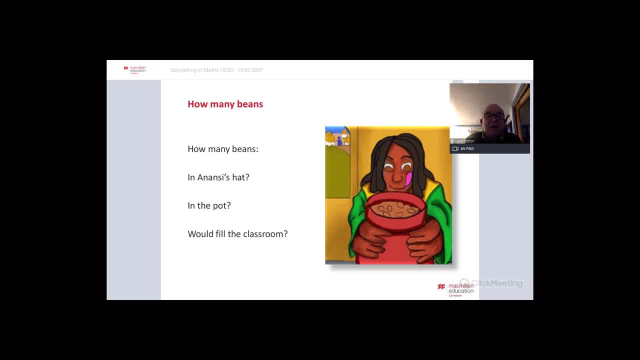 We can calculate beans: How many might be in a hat, How many might be in the pot, How many would fill the classroom- And I'll come back to that in a, in a, in a very brief moment. but we can start to think about volume using, using the beans. 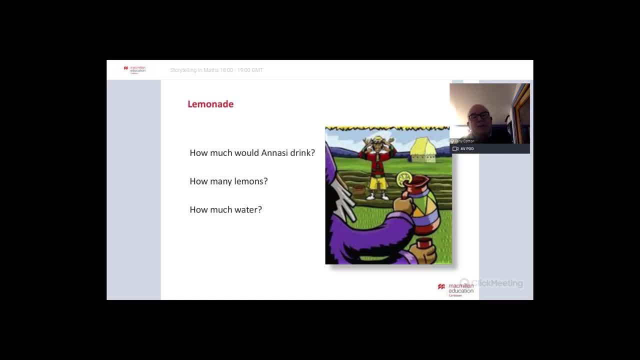 Halfway through the story, grandma makes Anansi some lemonade. We can start to think about recipes for lemonade. What would we do if Anansi had friends helping him? What would we do if we're making lemonade for all of our- our class? 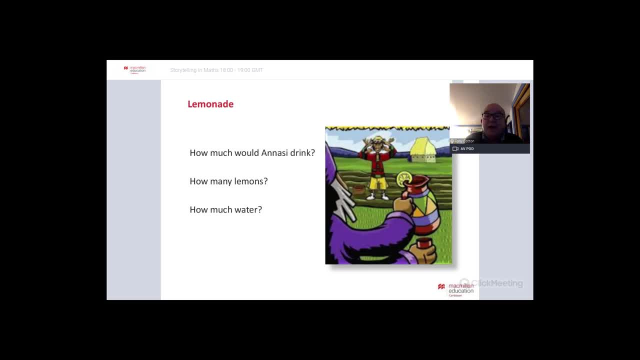 What's the ratio of lemons to water? How much lemonade would Anansi drink during the day if he drank one glass every hour? Those sorts of questions. I'm thinking of trying to do this with a, with a group of kids. 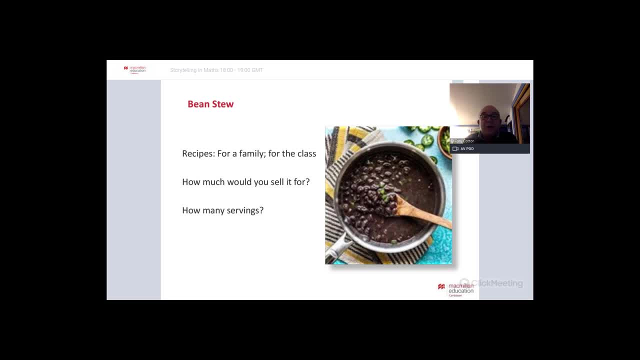 It's a school near me and on the end of the activity we'll be making a bean stew for the parents when they come and collect everybody, because that will need to think, we'll need to think about recipes and we'll need to think about servings and we'll need to think about how much we'd have to spend and how much we might sell it for. 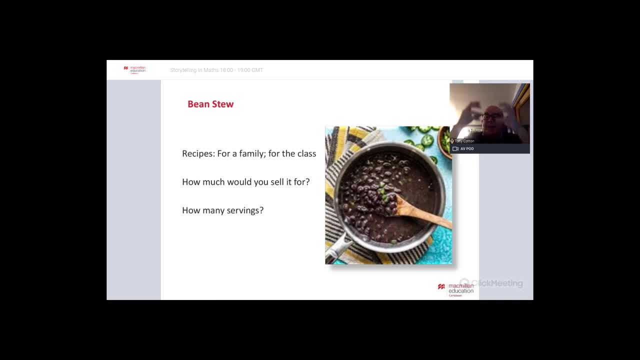 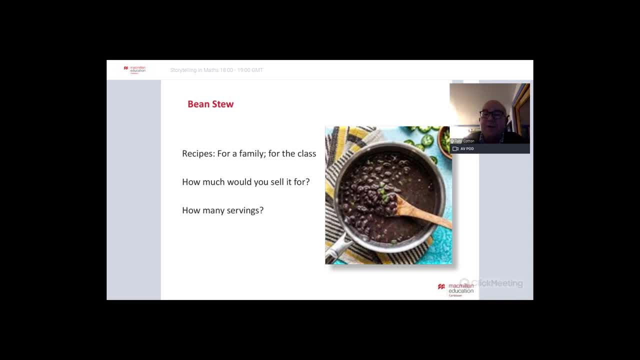 All sorts of ideas come to mind. All sorts of ideas come to mind. All sorts of ideas were were flashing into my head of different ways that we could, we could use it mathematically And I thought, well, is it just because I've chosen an Anansi story? 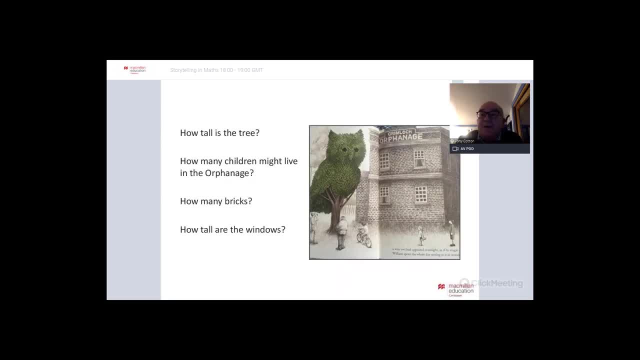 So I wanted to look at the book that my grandson was reading, and he was reading a book called The Midnight Gardener, And that's the page. that's a page out of The Midnight Gardener which I just opened up at random. And again, I looked at that with my mathematical hat on and started thinking. 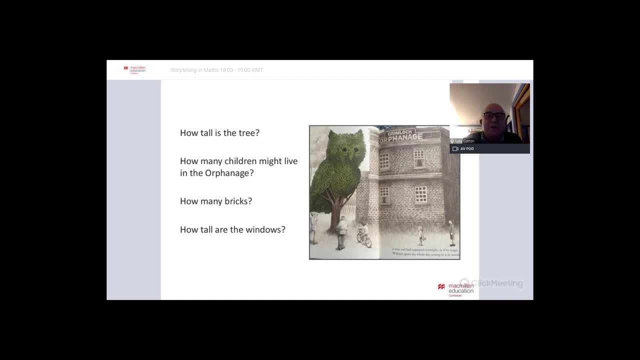 And again I looked at that with my mathematical hat on and started thinking: Oh what? what questions might there be? I wonder how tall that tree is. I wonder how many children are in the orphanage, because there's at least four bedrooms I can see. 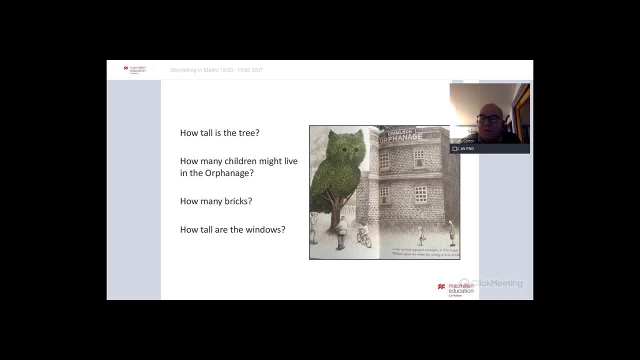 So how many children might I wonder if they sleep in bunk beds or or or single beds? I wonder how tall the windows are. I wonder how many bricks there are in that, in that wall that we can see. So how many bricks will there be in the whole orphanage? 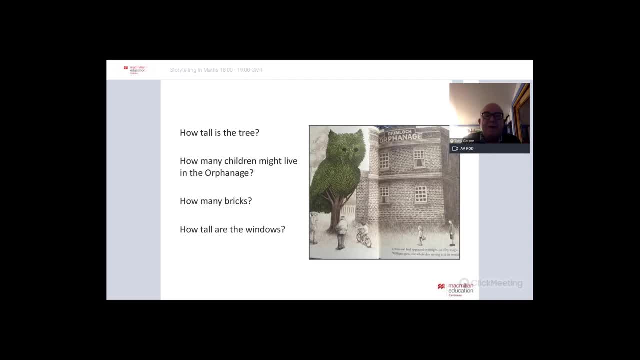 So suddenly there's all sorts of of mathematics that come to mind. It came out of that And again I I worked on this with Felix. All we asked those questions and I said: how tall is that tree then? And he said: well, it's the same size as the orphanage. 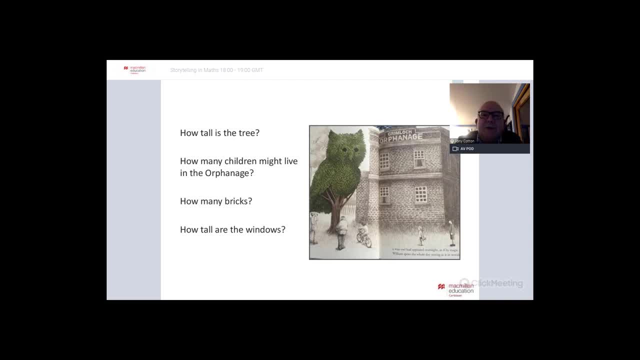 So I said, well, is it bigger or smaller than our house? And he said, well, it's bigger. I said: how do you know it's bigger? Well, there's more floors in the orphanage. So he was starting to. he was starting to to look at that picture in a in a slightly different way. 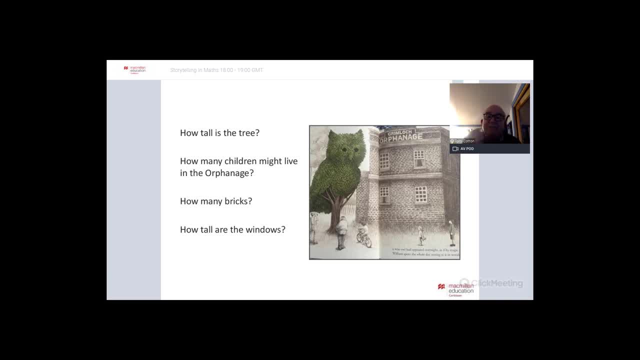 That's right. And how big? How big might the windows be, Charlene? and if, by working from the side and we can use the size of the children to think about the size of the windows and one of the ways that we we use the size of the people to think about how big the tree is? 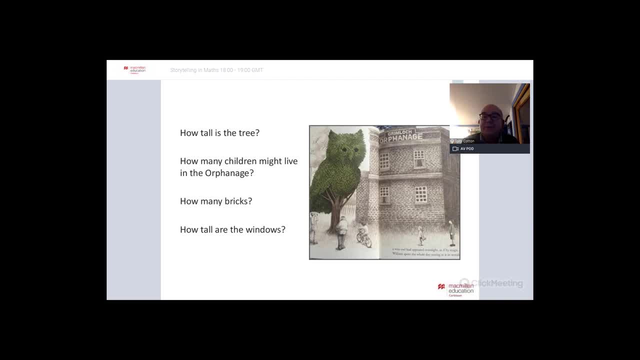 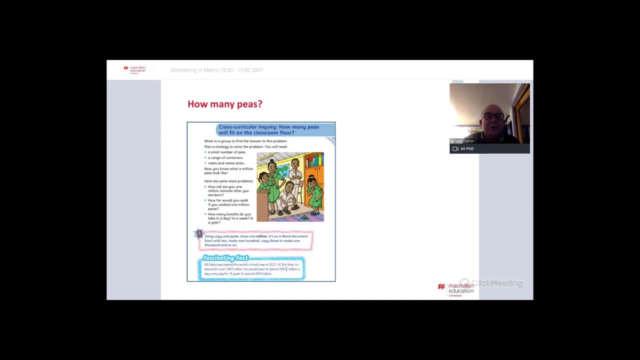 So suddenly we're starting to do all sorts of of mathematics Again. those of you that were here last time remember that as I used examples from the explore mathematics books I'm in in Jamaica, that I've written in in Jamaica, that I know Kingston bookshop in has to show you how the real world could come into into mathematics. 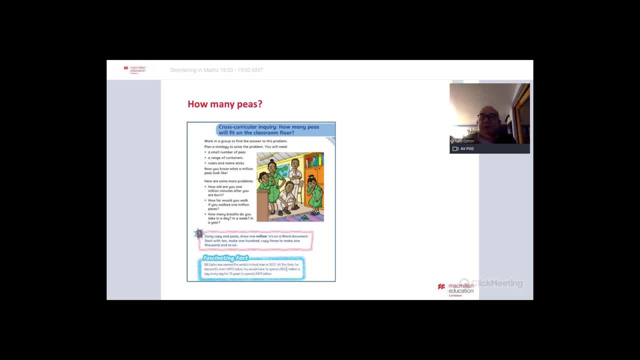 And here are some examples of how these cross-curricular inquiries can build on the sorts of stories that I've been been talking about. So the first one is thinking about the P's. If we've, if we've done that Anansi story about P's, we can start to think about, well, how many P's would fit on our classroom. 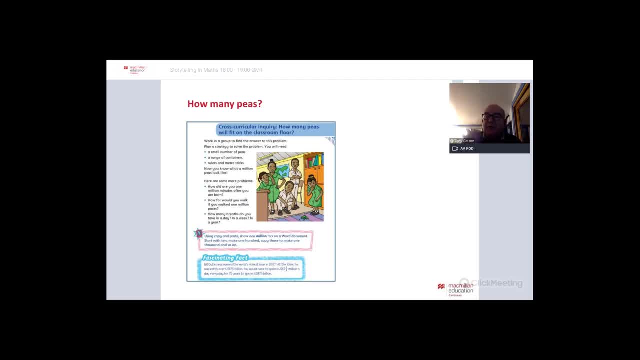 For example, If we've done that Anansi story about P's, we can start to think about how many P's would fit on our classroom- And of course we don't literally put P's all over the floor. We might fill a one foot square outline with P's. 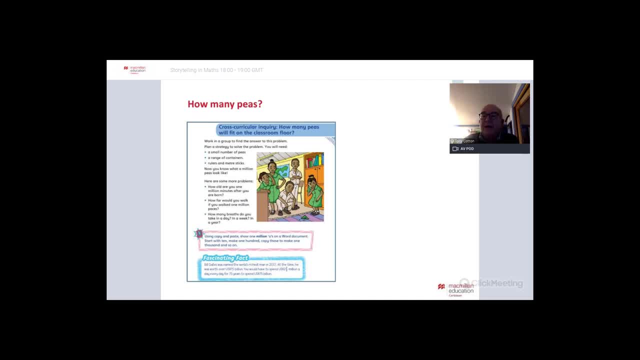 And then we can multiply that, multiply that up, And of course we don't literally put P's all over the floor. We might fill a one foot square outline with P's and then we can multiply that, multiply that up. Thinking about the chessboard problem. 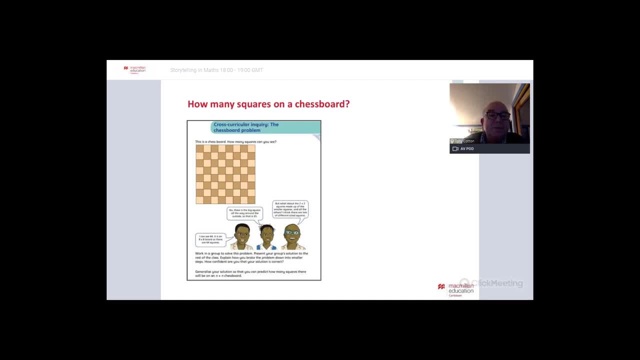 We can also think about how many squares are there on a, on a chessboard, And somebody asked and we can see there are 64 small squares. But if you look carefully you might start to see that there are quite a lot of squares made up of four small squares. 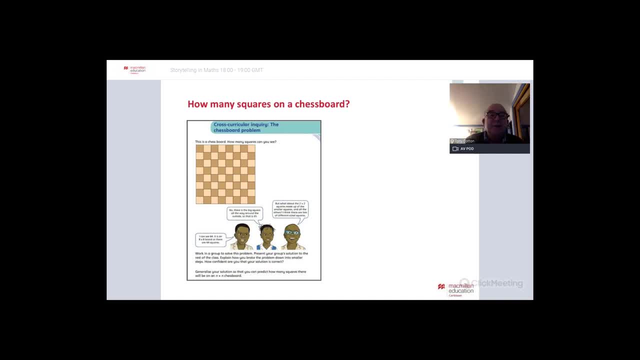 So squares that are two by two. There are also squares that are three by three, So they're made up of nine small squares. So you'll notice that we're now starting to talk about the square numbers. So what we're doing is developing the idea of the chessboard problem and looking at it in a different way, coming from that same story. 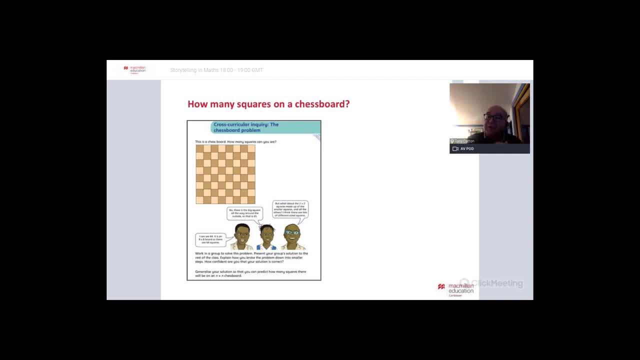 Somebody this afternoon talked about doing this on a geoboard, and I think that's a really good idea, because we can model the different squares on a geoboard And finally, sometimes another form of story or creativity might be doing a role play. 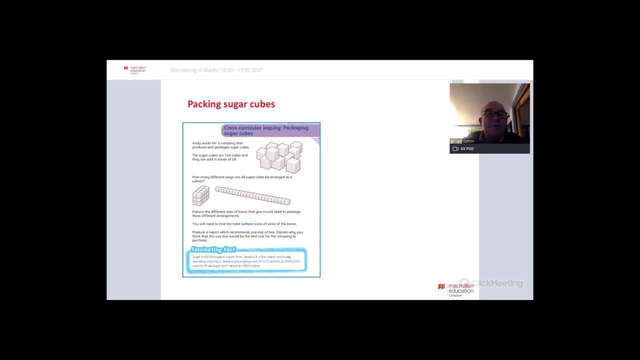 And this might be an example of how you could Use role play for mathematics. So what you can do in your classroom is form small groups, and they all work for a packaging company that's packaging sugar cubes, And their task is to work out the best way to package sugar cubes is: how many different ways can you pack 24 sugar cubes as a cuboid? 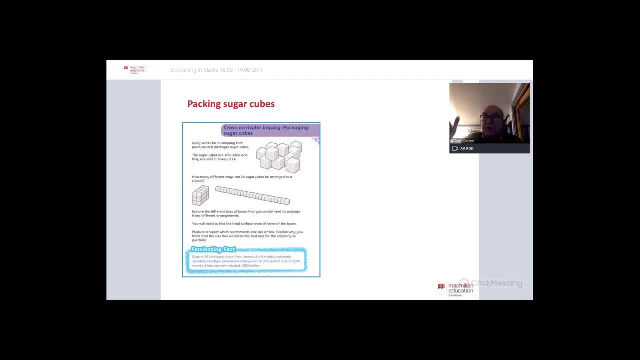 And which do you think the best way will be to pack them so that you can fill boxes efficiently? So we're still in the It's. if we're still telling stories, we're still being creative, but maybe that's a cross between creativity in the real world. 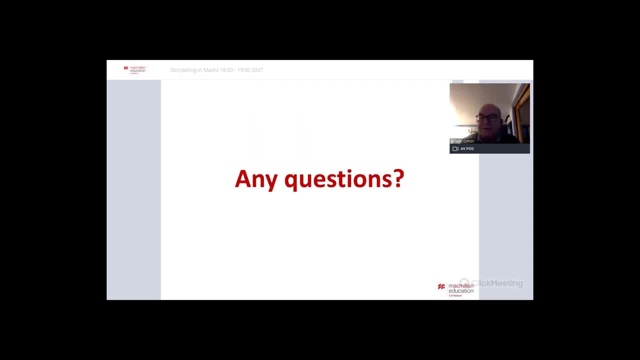 OK, so that's the end of what I've got to say. Then I'm going to take questions. sorry, I pause because I just saw in the cases question which I think is is a really really good question And And I've done some of 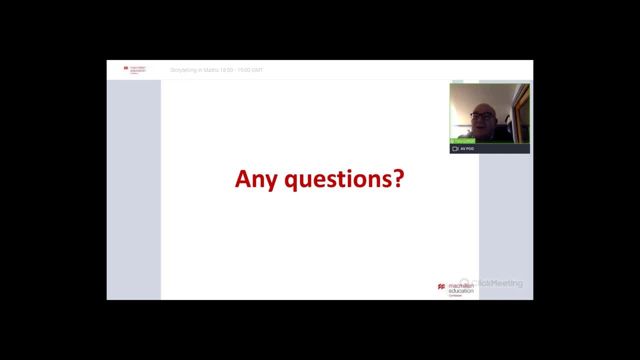 This with with three and four year olds online, and a lot of it is to do with asking them to find things or asking them to draw things and and show and show me things. So if we're thinking about the dot dot patterns, that's something that they can do and we can either show- show the children the dot patterns and ask them to show how many there are, or or get them to draw things. 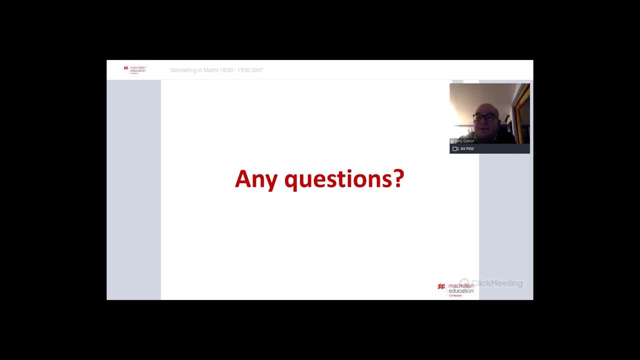 And Going and finding things is you is a really good, good, good way to to to involve children, children online and actually finding YouTube videos of the stories and sharing those. if you're using zoom or something sharing, sharing that through the share screen and you can share your images through through through share screen. 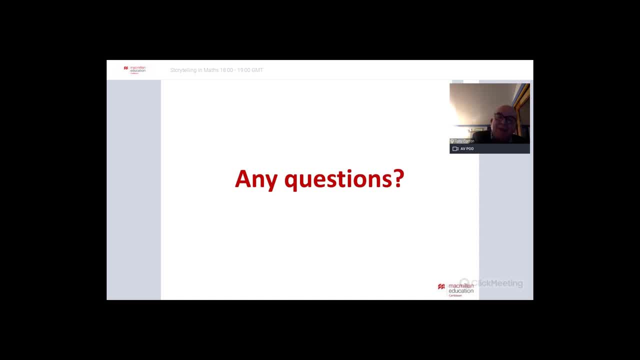 And another thing you can do- and obviously it depends on the parents of the children- is set them a task to do That the parents can, That the parents can then take a photograph of, upload and send it to you later, which you can then use the next day. 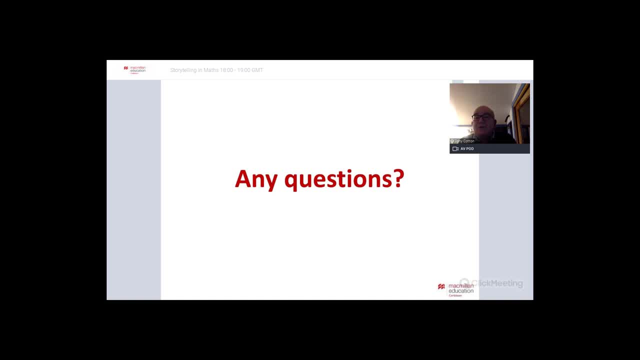 If students can't read, then you're. we read stories to students, students who can't read that way. So So it's just exactly the same. We did, We read the stories like I read the Nancy story to you, And the story is still, is still engaging, I think. 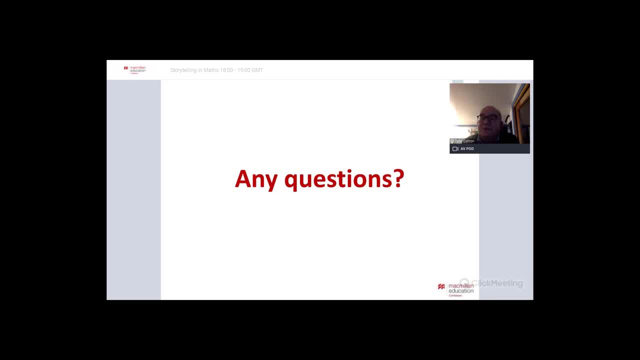 So somebody else asked me. I noticed a store, a question coming through which was about engaging Boys in mathematics, and I think one of the ways of doing that is finding the stories. I've often found that boys really like the Nancy stories. 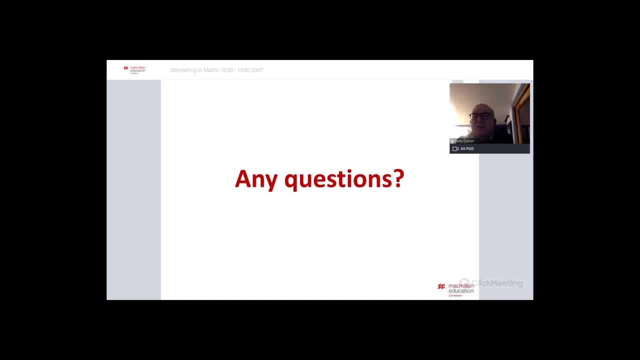 Actually, I think they like the cheekiness and the naughtiness of a Nancy, But find the find the stories that the boys like and draw the mathematics out of those stories. Exactly, Kerry, Yeah, And that's just what I was saying, Joel. 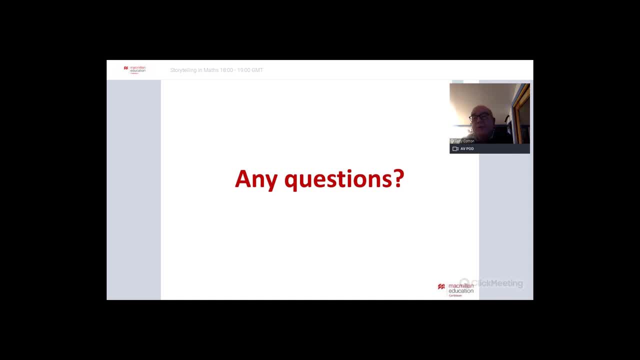 I think that you will know The stories that your children love and you will know the stories that the parents of your children read to them and you will know the folk tales that they that they know. And one of the things that I started doing now as a result of researching for this webinar is I'm building up my own kind of catalog of stories with the mathematics that I can draw out of them. 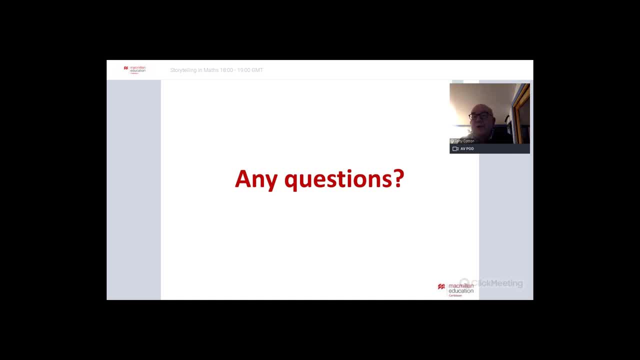 So what I do is start with a good story. I don't start with the mathematics. I start with a good story and think of what's the what's the what's, what's the math that come out of that, And eventually I will have a catalog of all the different mathematics in the story I can use. 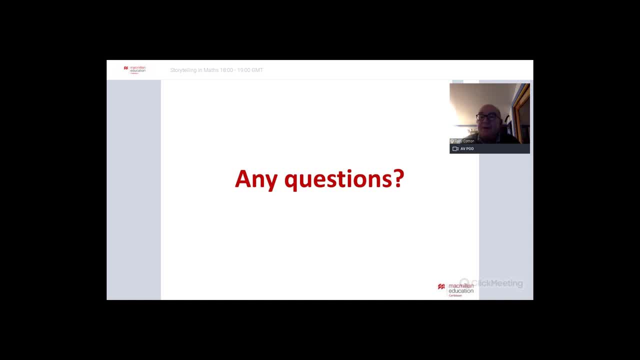 I think that one about announcing the pot of the beans stew is all about volume. When you start to think about the lemon lemonade and how many glasses of lemonade Mikey drink, how how deep is the pot? How much stew can he fit in the pot? 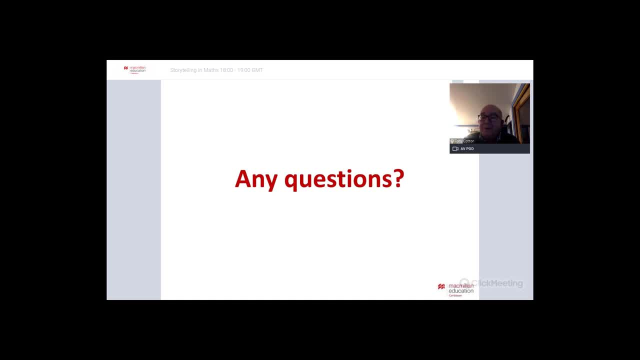 How many beans would fit in there would fit in the pot, And so, yeah, I think that one ties ties directly in with with volume. Rona, give it a go. Read them that stuff, Read your children that story and work on, work on volume with them. 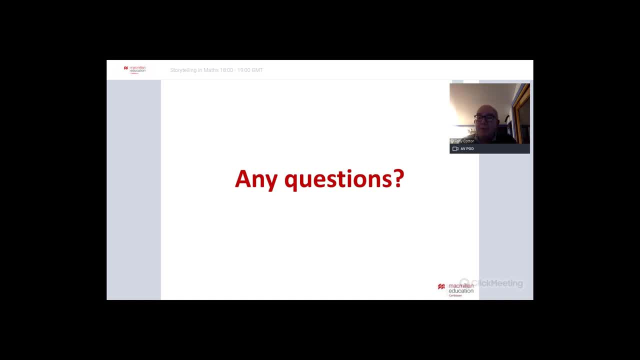 Bring in a lemonade bottle, Bring in different pots of stew, Compare, Compare the, the volumes. There was a suggestion this afternoon about making lemonade and having the having different glasses that Nancy might choose to drink the lemonade out of and Showing that it's called conservation of volume. 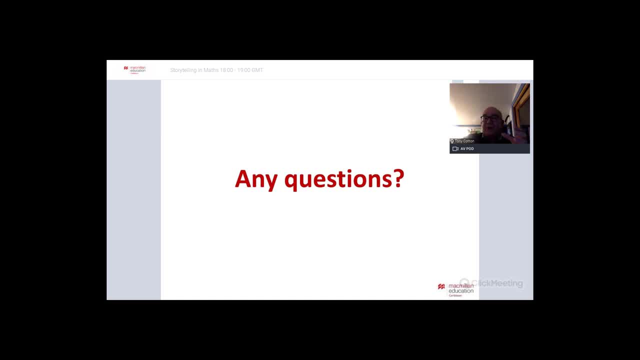 When you pour the same amount of lemonade in different shaped containers, it doesn't come up as far Any more. any more questions. Absolute pleasure, everybody. Like I said, I just wish I was with you all. I think we'll leave it there, Tony. 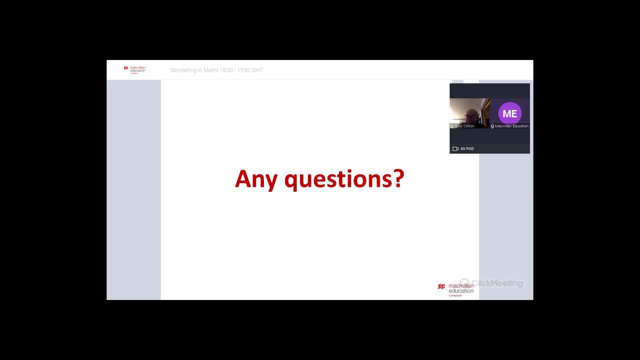 I think most of the questions have been, So. thank you so much to Tony, as always, for a fantastic session, and I hope that the attendees enjoyed some of those stories, And I can see from the feedback that trying to implement this and trying to get students- both genders- involved would be really, really great. 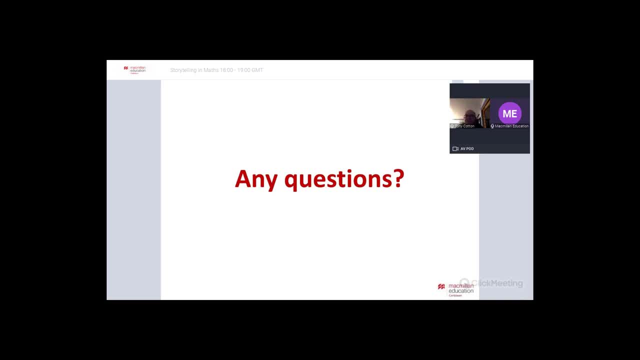 So thank you so much, Tony, Thank you to the attendees And just to let you know, Tony will be hopefully delivering sessions for us, if he agrees to this, in the upcoming months. So that would be really great. So we will let you know once we start. 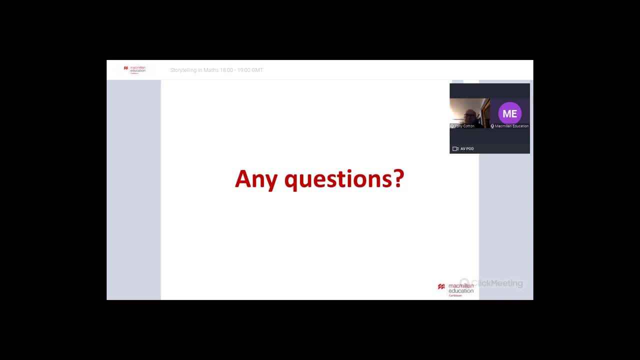 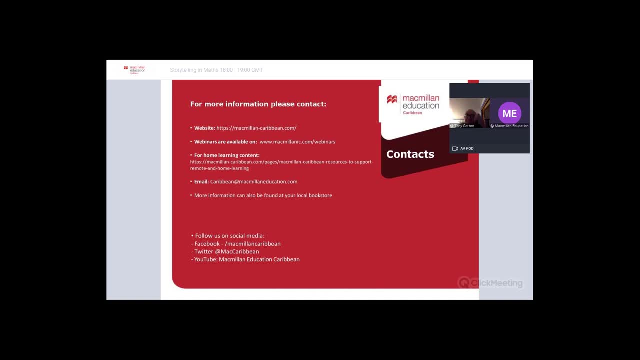 I'm planning our next set of webinars and we will let you know in due course. So just before you go, a bit of information. the webinar recording and the PowerPoint presentation will be sent by email within two weeks. The CPD certificate will be automatically available as soon as the webinar finishes. 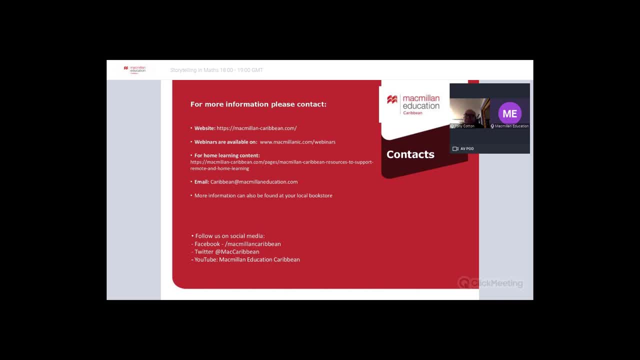 And do follow us on social media and do email us if you have any questions. So thank you again. Take care, Stay safe. We look forward to seeing you soon. Thanks everybody. Thanks for being so active. We'll see you in the chat. Bye.